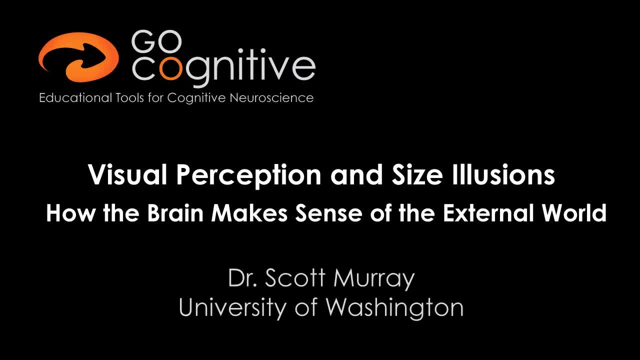 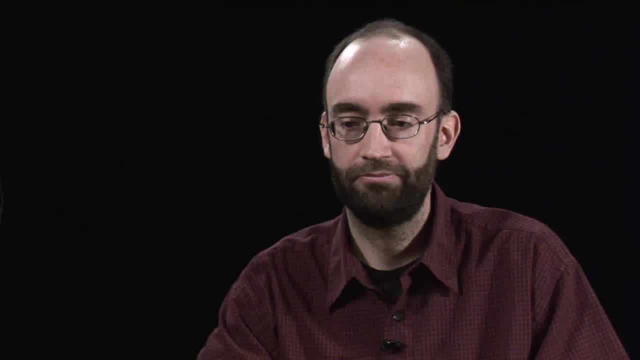 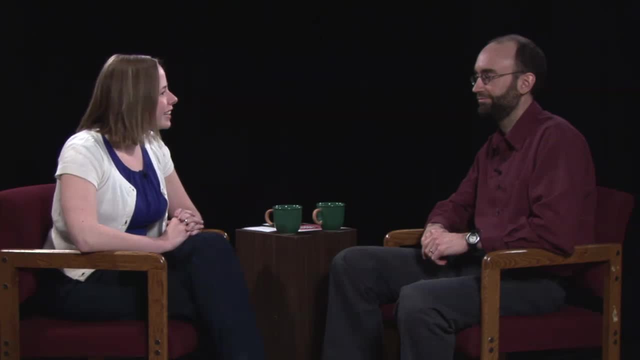 Hi, I'm Kylie Pfeiffer and lucky enough to be speaking with Dr Scott Murray from the University of Washington today. He studies the neurological basis of visual perception. Dr Murray, thanks so much for taking the time to be with us today. 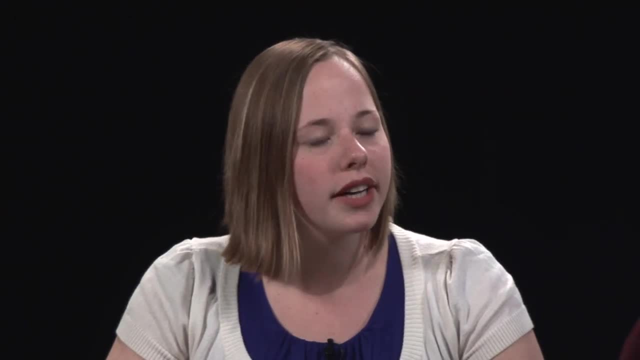 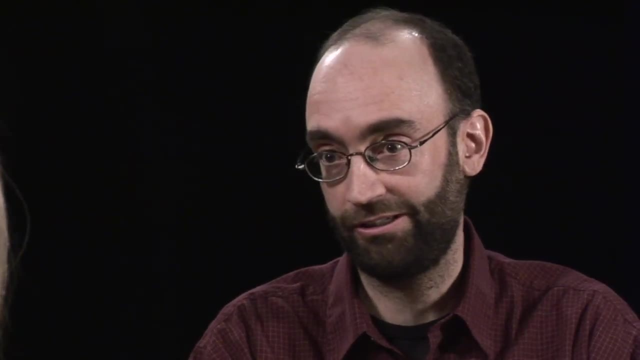 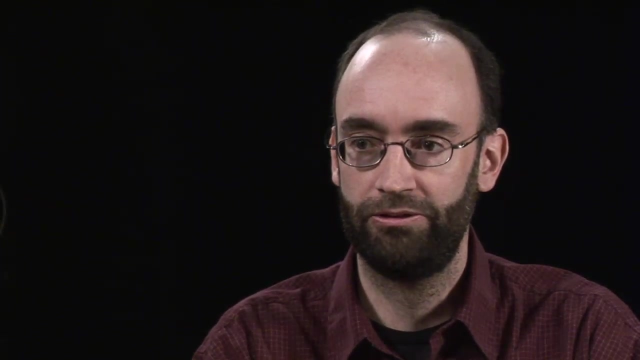 Thank you for having me. So could we start out by you just walking us through the steps of visual perception and how that works? Sure, First light enters our eye and gets transduced by our retina. Then from the retina it makes visual information travels to the cortex, It makes one stop in a structure called 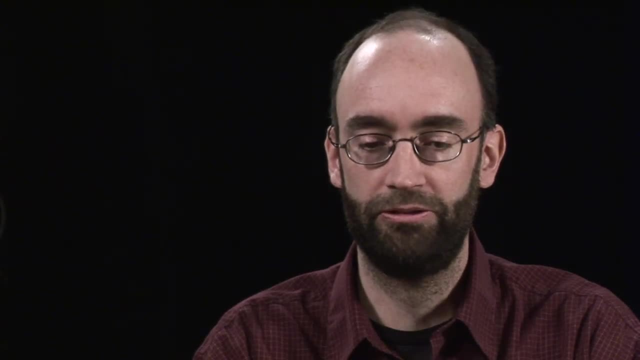 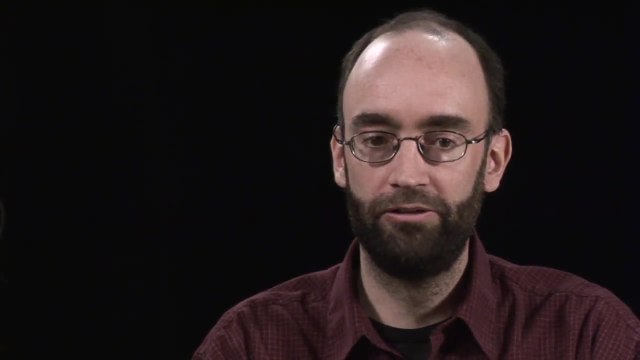 the lateral geniculate nucleus in the thalamus and then projects directly to the cortex, to an area that we call V1, or primary visual cortex. Then from V1, visual information travels to other visual areas within the cortex labeled V1.. 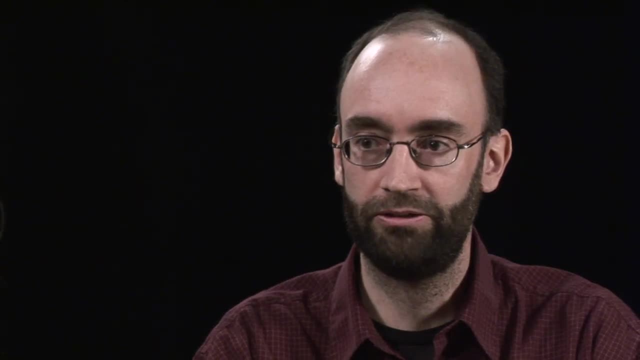 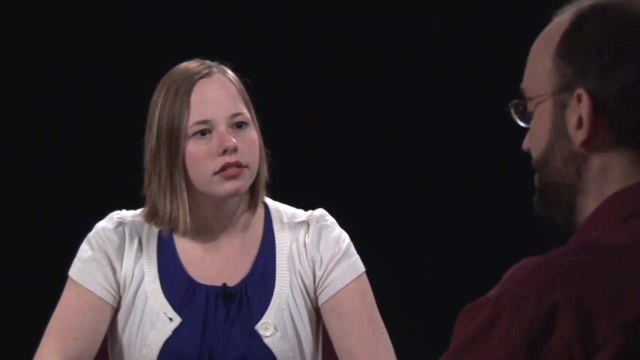 V2, V3, and up into the parietal cortex and also down into the temporal lobe as well. So where then does perception start in that pathway? That's a really good question. So if there are upwards of 30 different visual areas, 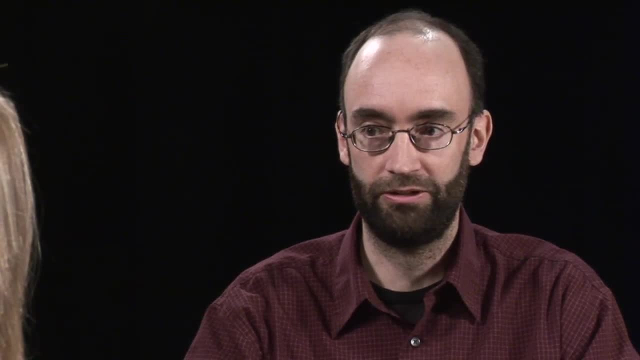 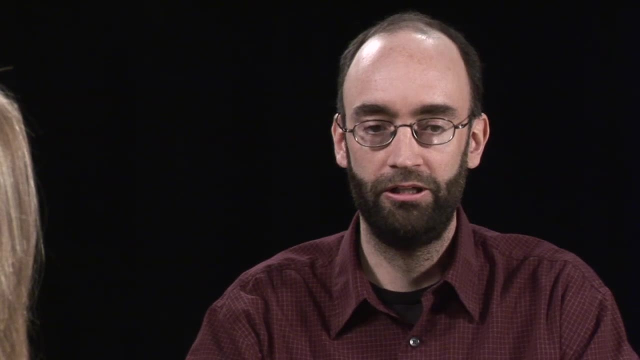 I think it's fair to say that not any one of those areas is exclusively involved in perception. It's probably a complex interaction between all of those different areas. It really depends on exactly what is being perceived. So, for example, we have specialized areas. 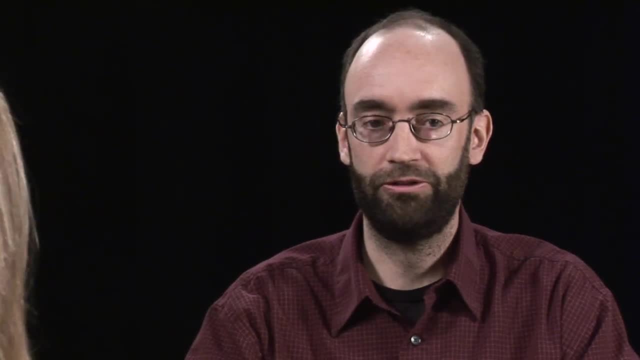 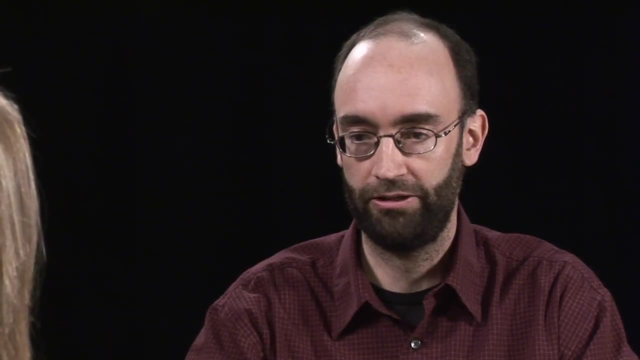 of the cortex, That process say motion. So if it's motion that's being processed or perceived, that particular area or group of areas is going to be highly involved. Similarly, if we're perceiving things like faces, areas that are specialized for processing that kind of information- 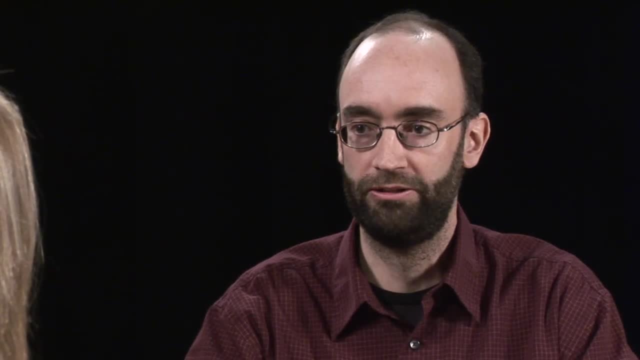 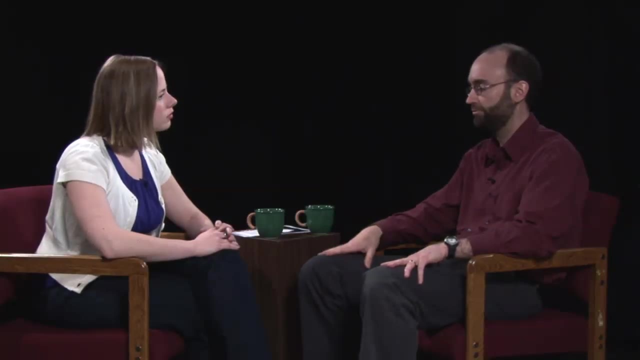 are going to be involved as well. So it really depends on the kinds of information that are being processed, in terms of which visual areas are actively involved in perception, And so is all the visual information that's coming into our eyes present in all of those. 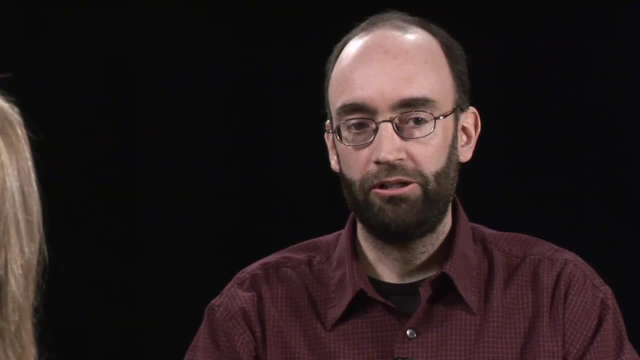 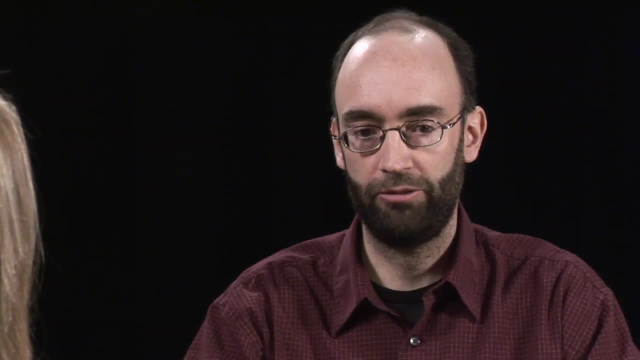 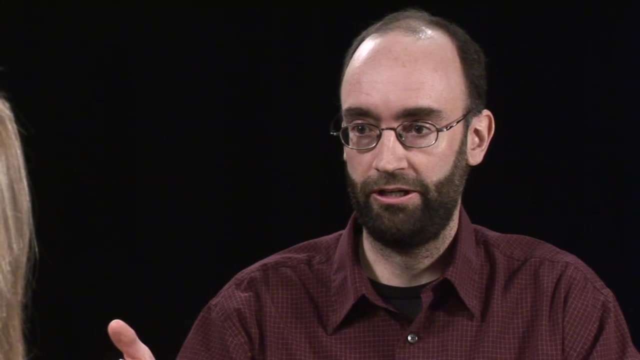 areas, or does it kind of get split up? Well, at least in the early stages of visual processing, it's likely that they're probably all equally involved in any given visual perception. But the higher visual areas, the areas that are specialized for specific kinds of visual information, whether it be faces or motion, 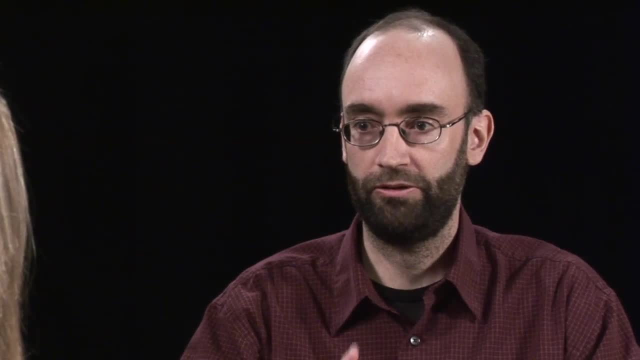 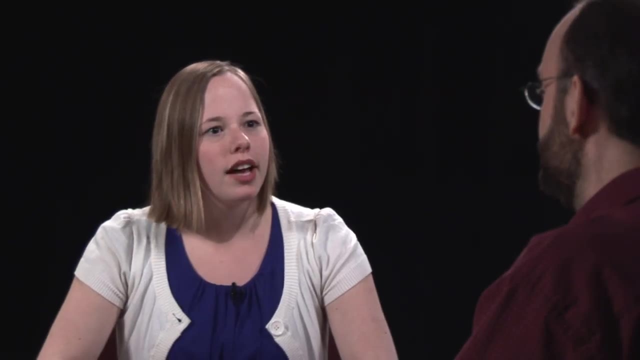 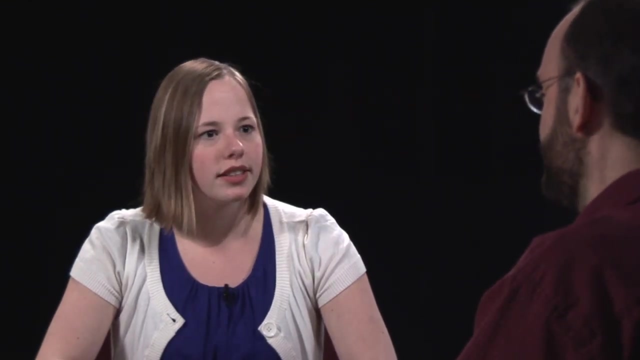 are fairly selective for the kinds of information that are present in an image. So information comes in through the retina and goes through the stream And I know that some terms in cognitive neuroscience are top-down and bottom-up processing. Where would you say that happens and what are those different functions? 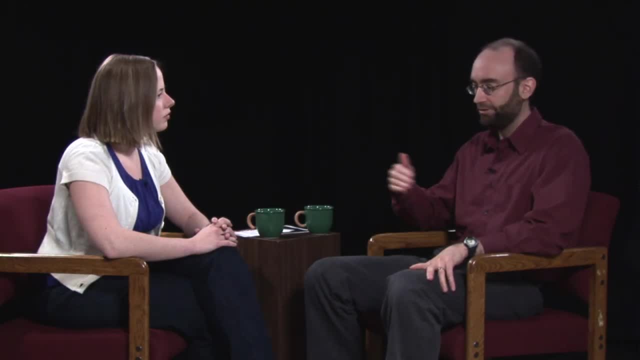 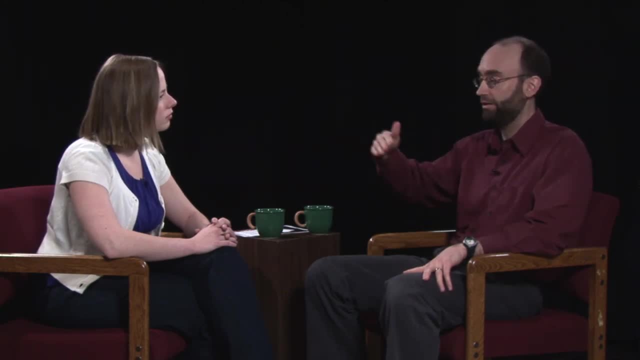 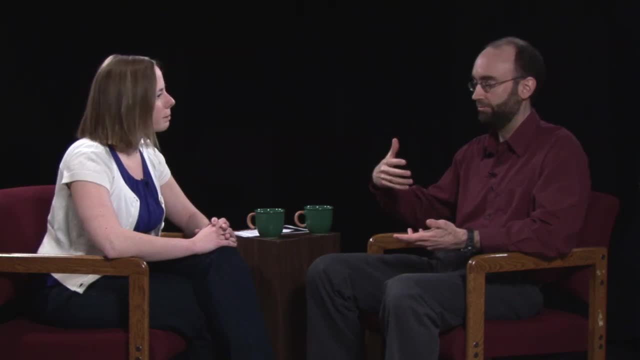 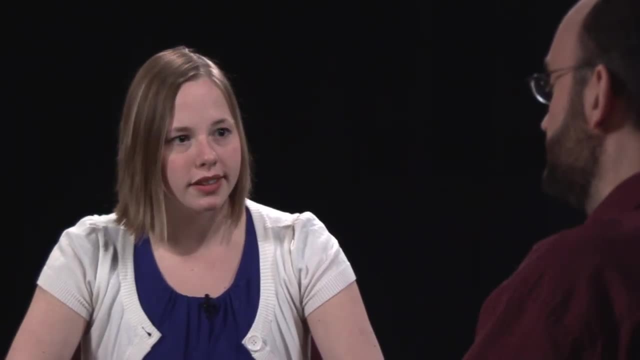 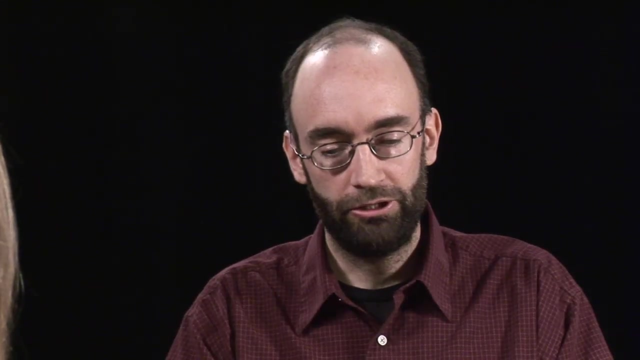 way also are connected in a feedback way, so that visual information can actually travel backwards through the visual system. So the term feedforward then refers to bottom-up processing. bottom-up processing and feedback is referring to what's known as top-down processing. that's exactly right. so, and in terms of what feedback processes are, 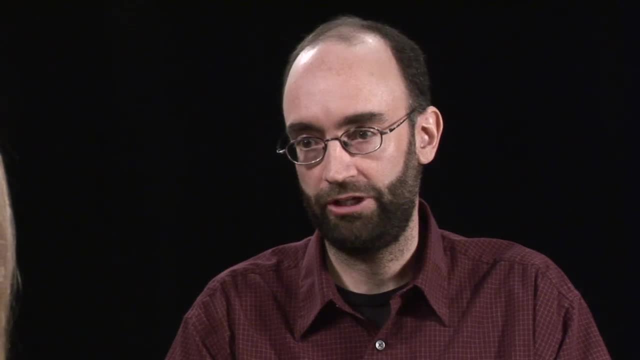 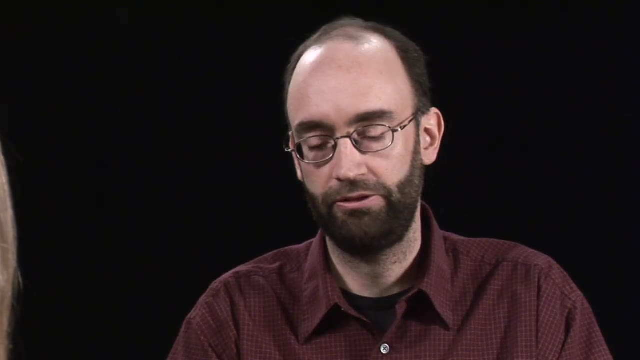 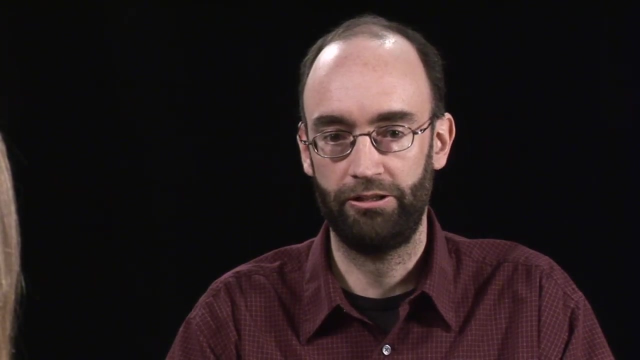 thought to be used for. one well-known example is visual attention, so we can modulate activity in lower visual areas through attention and it's thought that this- the feedback, is important for that. but in addition, feedback likely is very important for affecting sort of contextual modulations of activating. 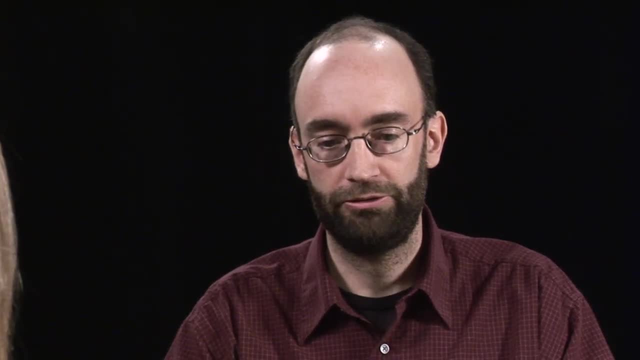 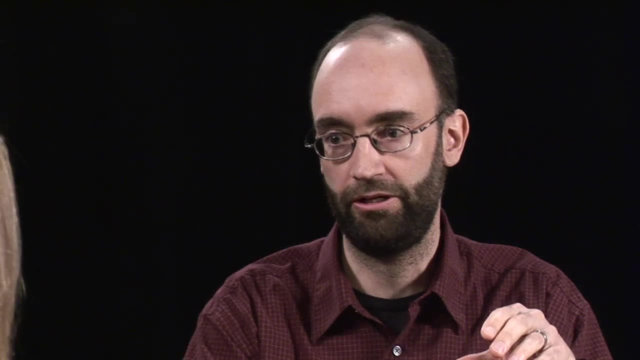 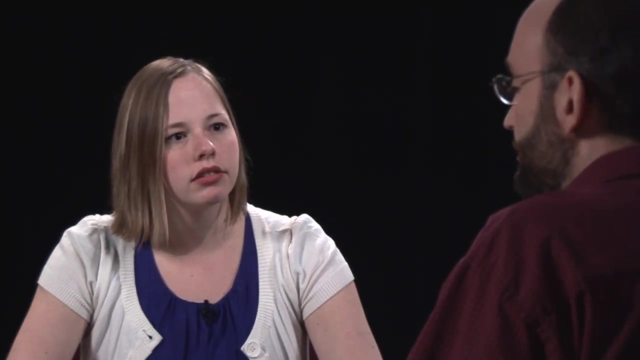 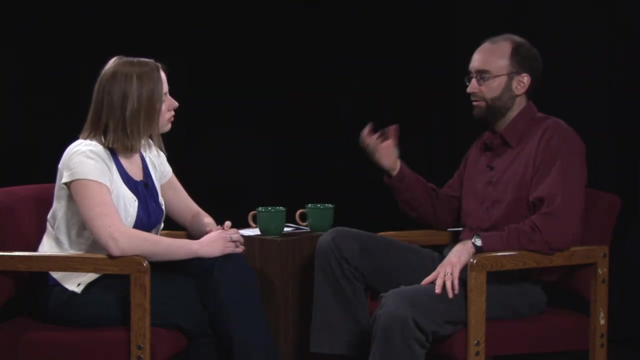 early visual areas. so surrounding information, for example, can have a large impact on the neural processing in early visual areas due to feedback projections. so then, what are the main characteristics of this visual processing? well, visual perception is often thought to be an attempt by our brains to characterize a pattern of light. 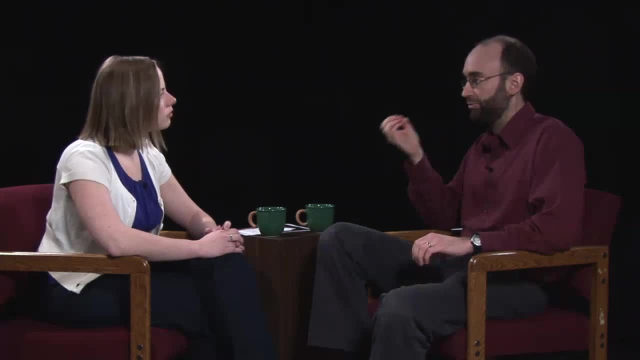 falling off your viene, even if it didn't separate the ground and anything falling on your vine, which is then prefer some the different types of light on our retina. that is, we want to try to measure precisely what's what's impinging on our retinas, but in fact is probably more accurate to describe visual perception as an attempt by our, our brains. 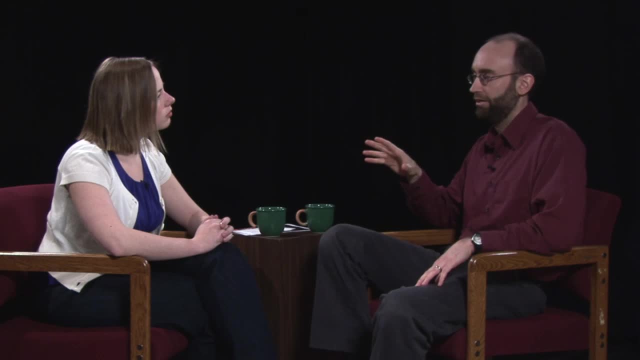 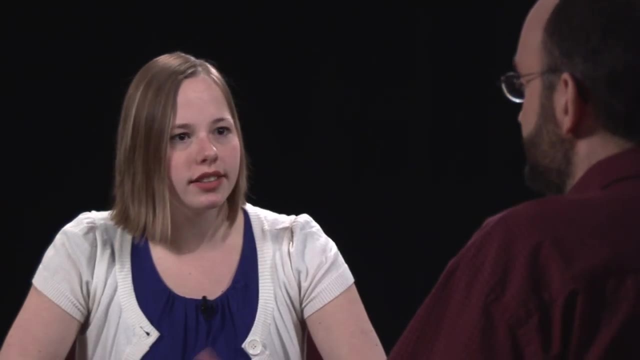 to figure out what, out there in the world, caused the pattern of light on our retina, and it's a really important distinction to make. so, then, is that a distinction between the distal and the proximal stimulus? that's exactly right. so the proximal stimulus is the stimulus that's actually. 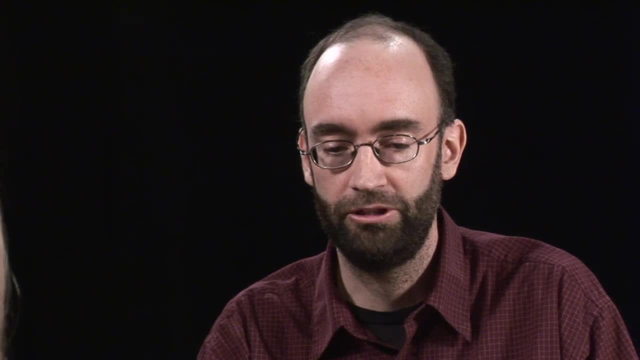 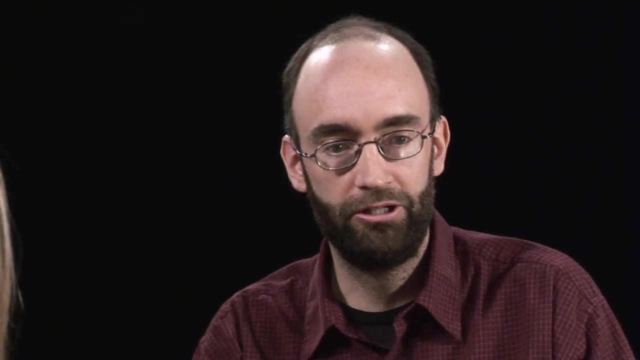 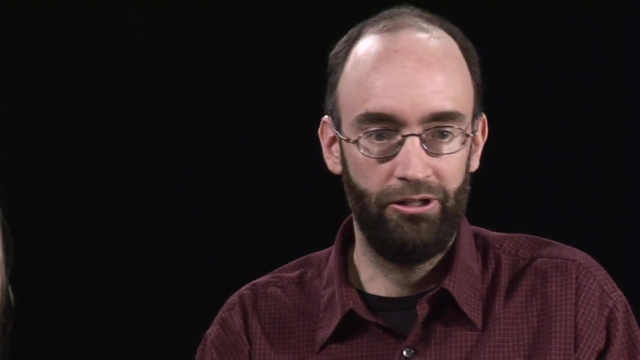 on our retina, that is the light impinging upon our visual system, and the distal stimulus is the thing out there in the world that caused the stimulus. that's really important to think about in terms of, say, brightness constancy, for example, so you take some object and could be a white cat. 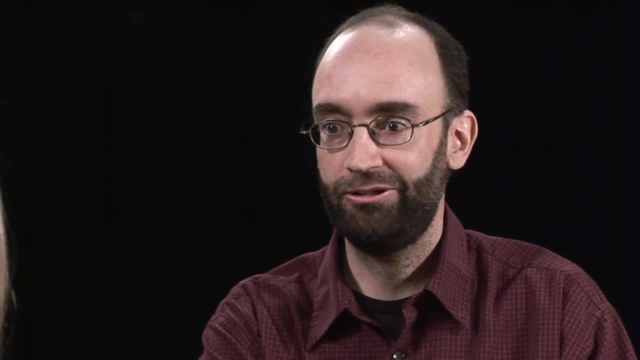 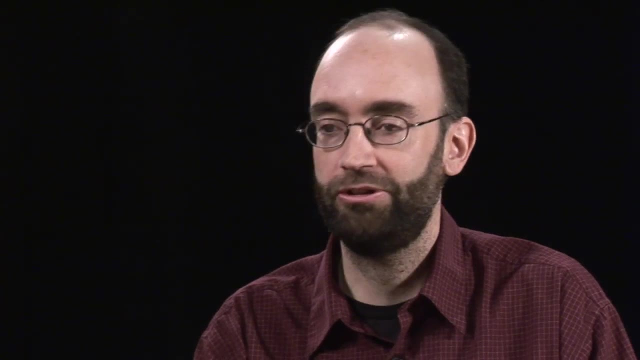 for example, out in bright sunlight, you take that cat, you put it in a shadow. the light, the amount of light reflecting off that cat is now equivalent to, say, a black cat, but you would still recognize that cat as being white. and so constancy has other forms too, in our 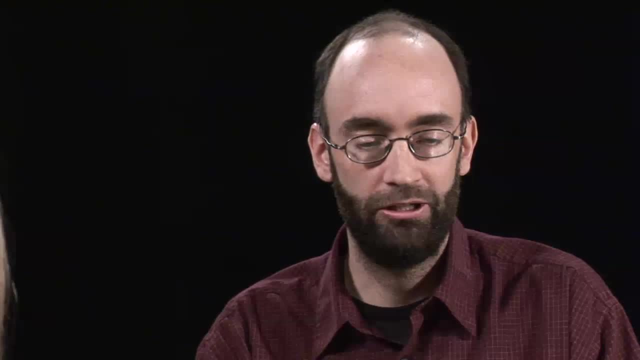 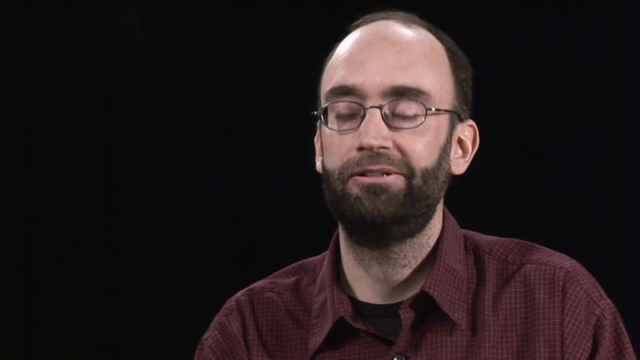 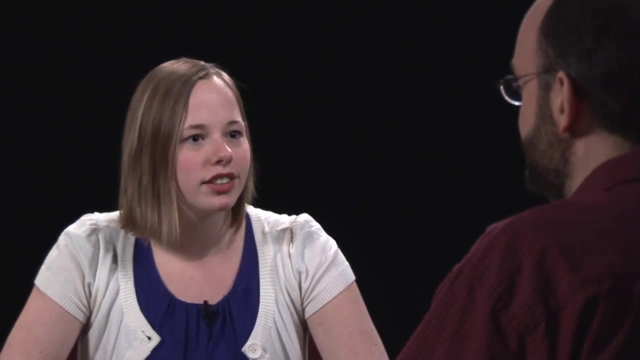 visual perception right, say, size constancy as well. if I stood up, you would recognize me as six feet tall, no matter if I was standing here or at the back of the room, even though the proximal stimulus was was changing exactly right. so how has our understanding of visual processing changed over? 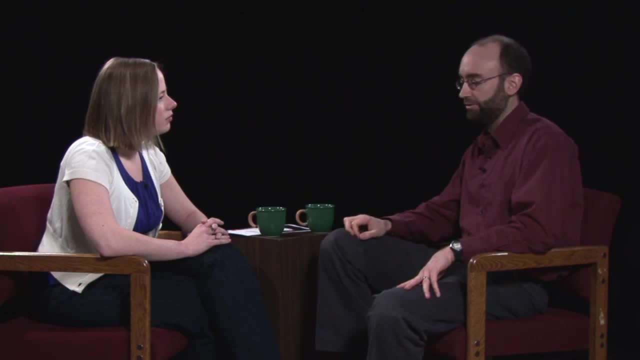 the years. well, from a neuroscience perspective, a lot of emphasis has been placed on the importance on really the proximal stimulus, that is, we. we we present a particular visual stimulus in an experimental setting and we ask how neurons respond to that stimulus, or what, what the fmri response is. 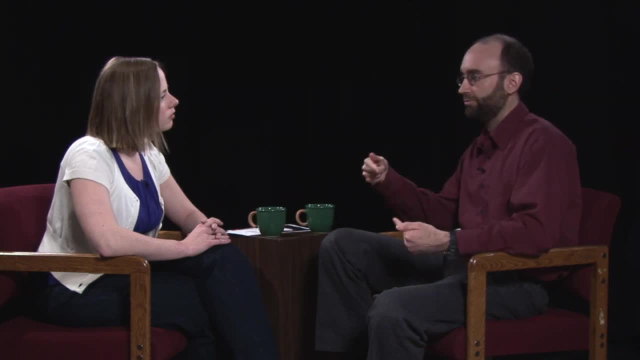 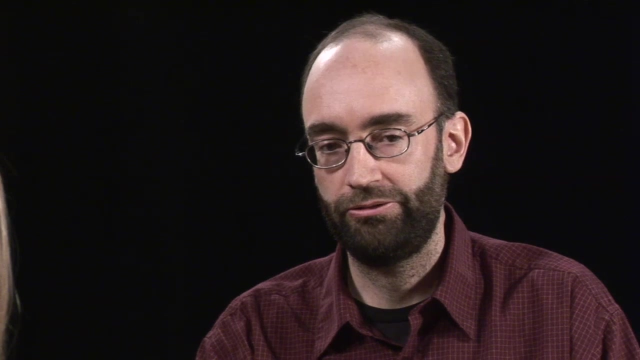 to that stimulus. but when we start thinking about the distinction between the proximal and distal stimulus, it becomes more appropriate to ask how the visual system transforms the proximal stimulus, that is, what's on the retina, into an understanding about what's out there in the world. so I think in the last five to ten years, 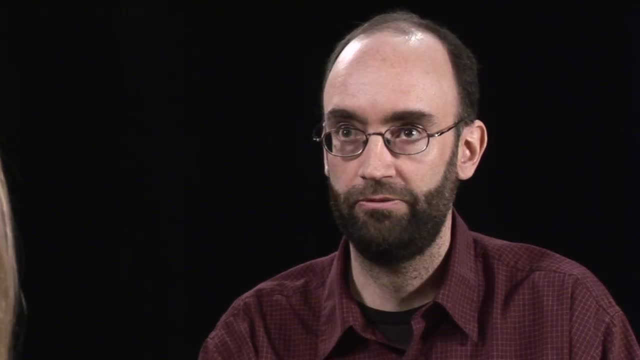 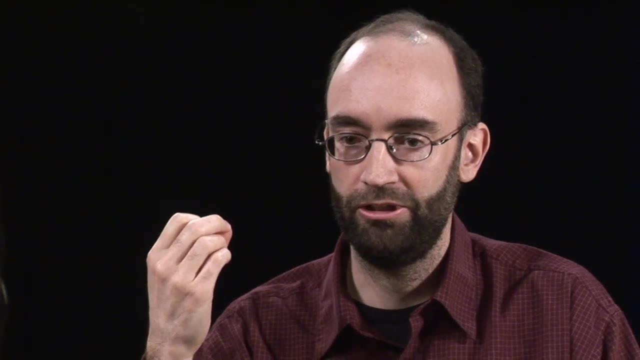 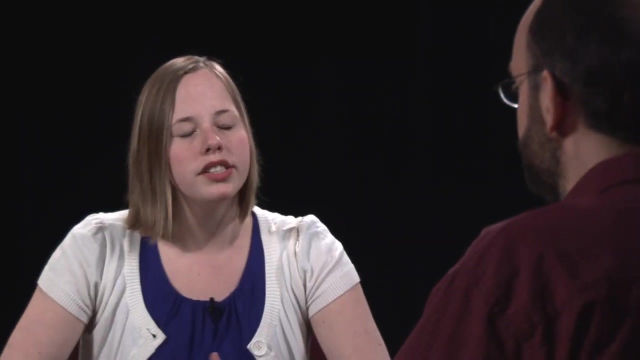 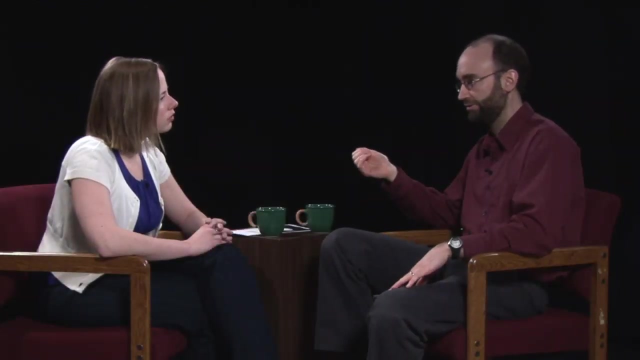 has been this increase in awareness of thinking about how that transformation occurs, from the actual input to the visual system, to its transformation to what's out there in the world and where is it thought that that kind of takes place? well, traditionally it was thought that that sort of transformation would occur in higher stages of the visual 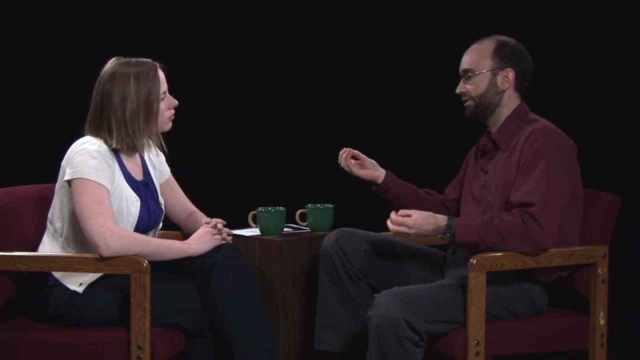 system that would code, for example, an object's identity. so early stages of the visual system were really thought to reflect the input at the retina at a very raw level, and what's starting to emerge now is this understanding that multiple visual areas, even very early visual areas, actually 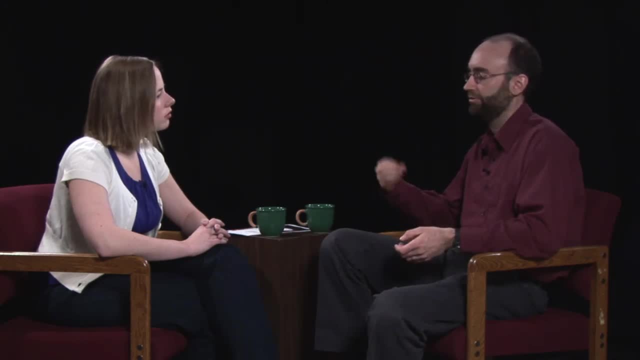 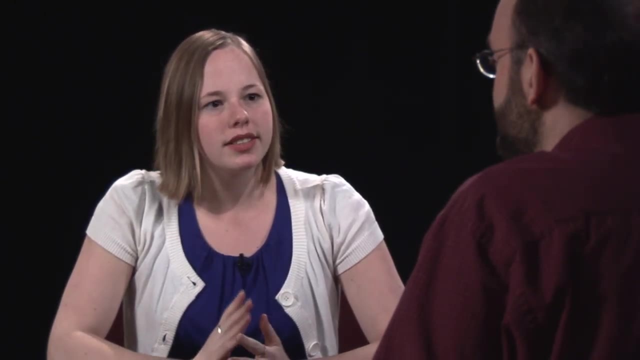 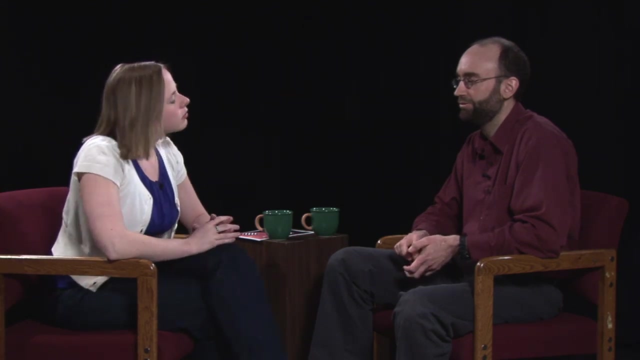 are involved in this transformation from the proximal to distal stimulus. so in most psychology textbooks they mention that this constancy happens in higher visual processing areas. is there any evidence that it happens earlier? there is actually, so I've been doing some recent studies looking at size constancy. so, for example, if you have two 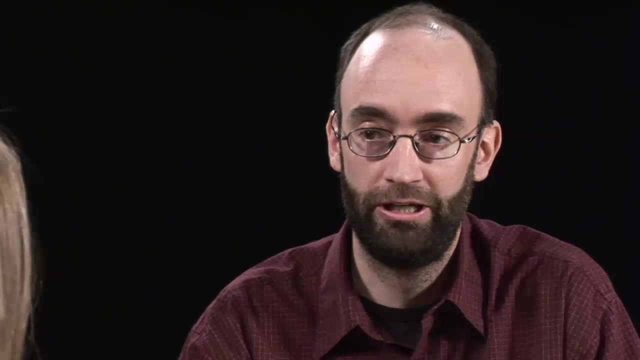 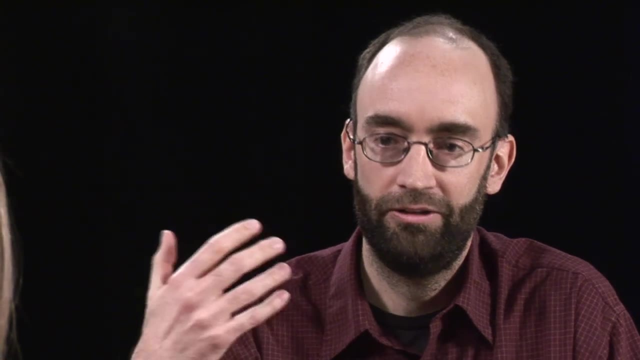 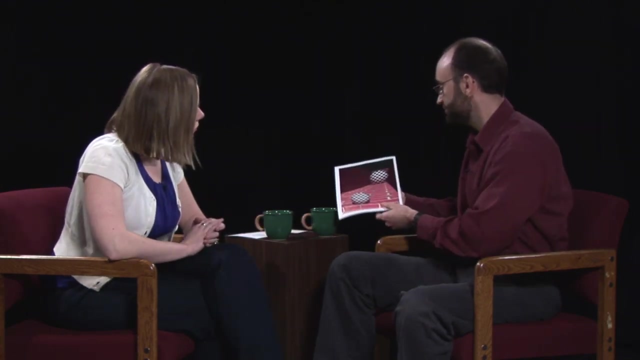 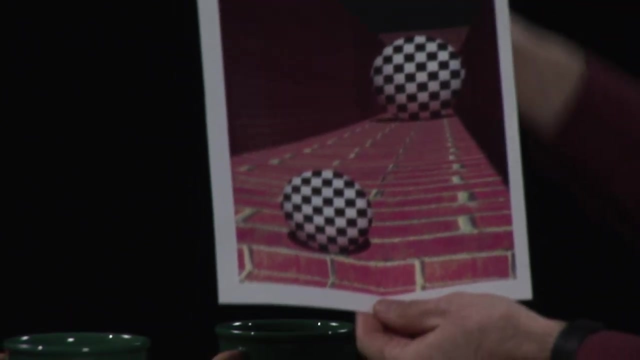 objects and one is perceived to be further away than another, but they actually project the same image on your retina, same size image in the retina. you perceive the one that's further away as larger than the one that's closer. for example, in this example here, what we have here is just a simple hallway scene, and these two spheres are exactly actually the. 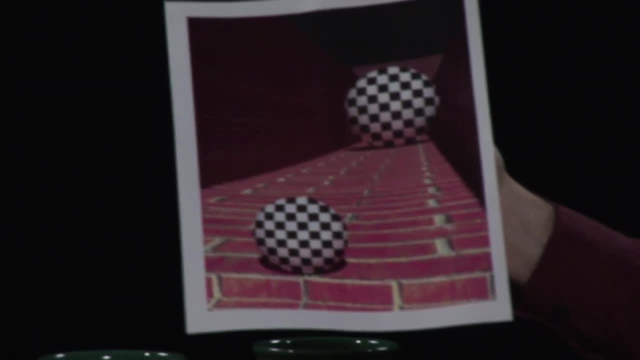 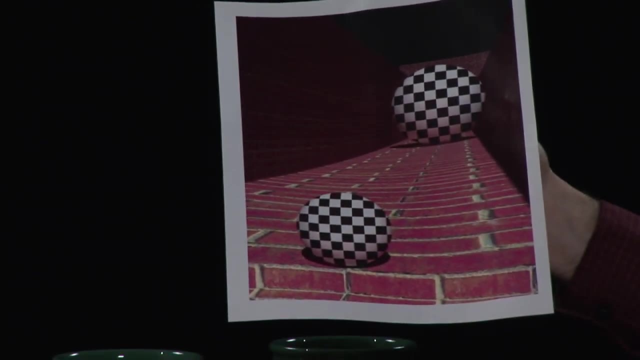 same physical size. they occupy the same number of pixels on the image, have the same retinal projection, but almost everyone perceives this sphere that's perceived to be at the back of the hallway is larger than the front of the hallway, and so what we've been able to do 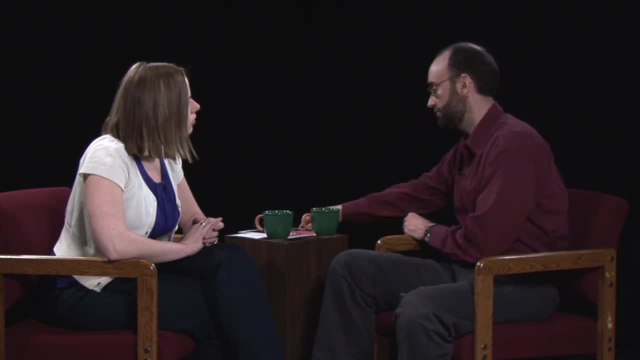 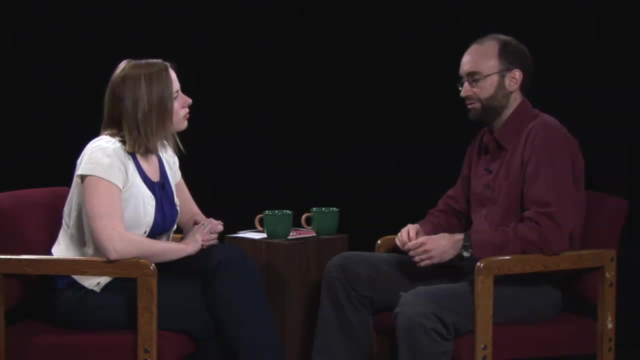 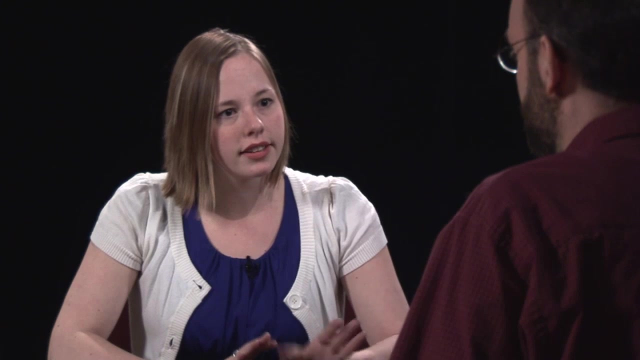 with this information and with using fMRI, is measure the retina topic maps in early visual cortex. so early visual cortex has this sort of convenient organizational structure such that nearby areas of the retina projected nearby areas on the cortex and that's what's meant by a retinotopic map. 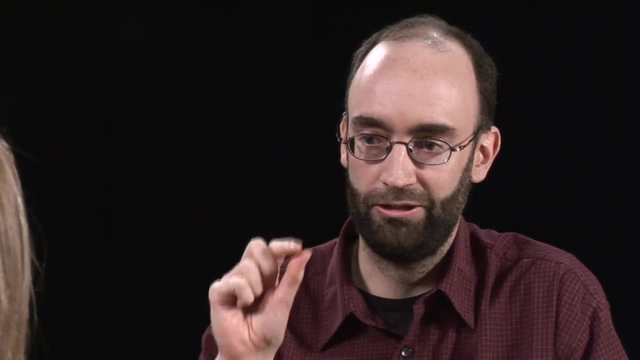 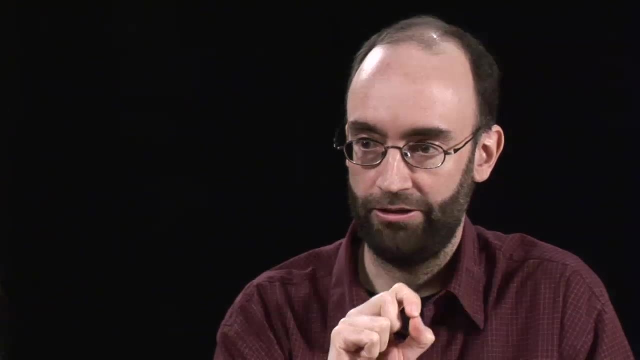 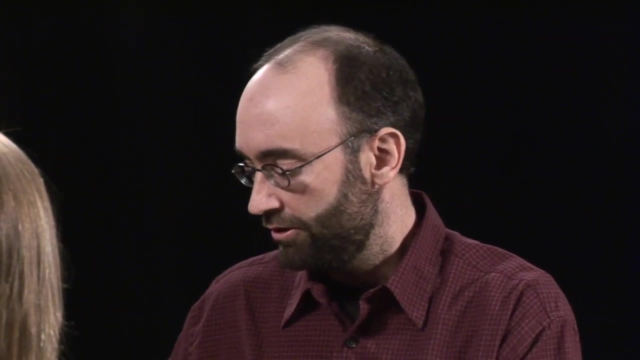 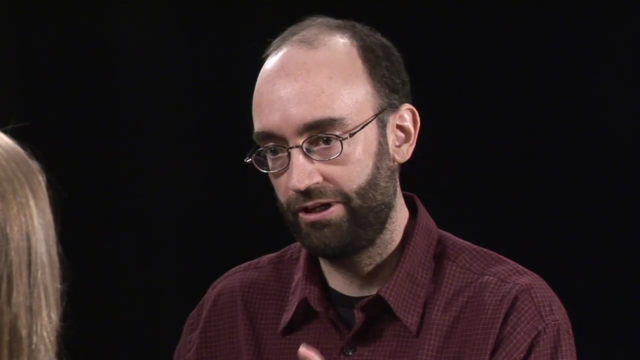 correct, that's right. so, for example, if you were to keep your eyes fixed and I shine a very small focused light on your retina, focused area, on your visual cortex, So, for example, with these images here, each one of these images is going to activate a portion of your map and we can compare the size of 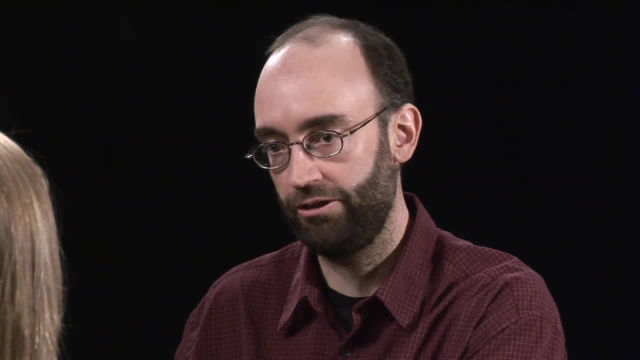 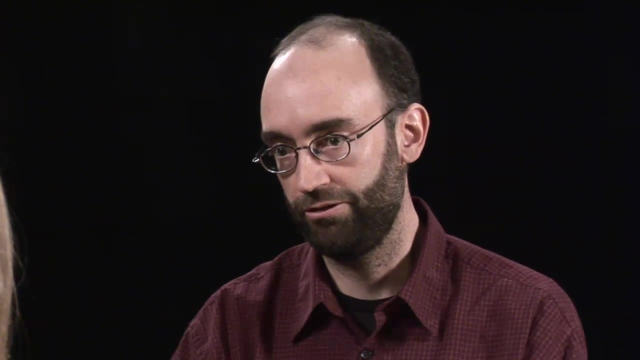 the area activated to the front sphere versus the back sphere. Now, based on the traditional way of thinking about the visual system, that these early visual areas just represent the retinal information, because the retinal information is equivalent for those two spheres, you, 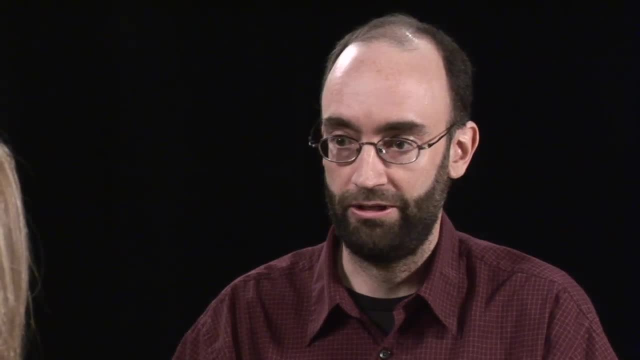 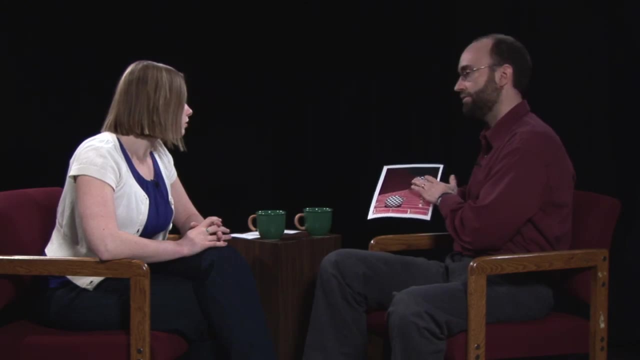 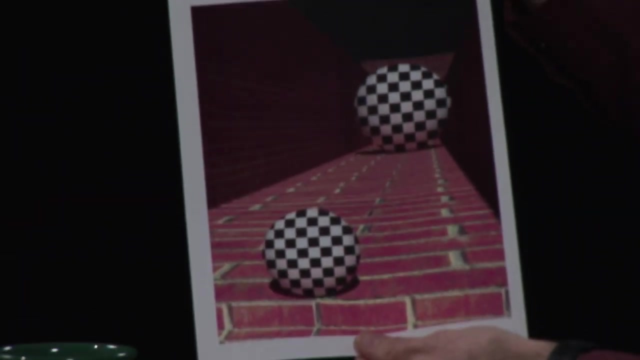 would expect that the representation in early visual areas would also be equivalent, But actually what we've found is that the back sphere actually activates a larger area, even in the very earliest stages of visual cortex in B1.. Really, It's important to realize, though, that the context in this particular image, the 3D structure, 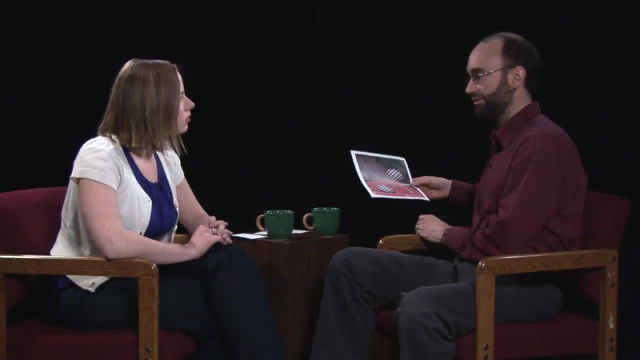 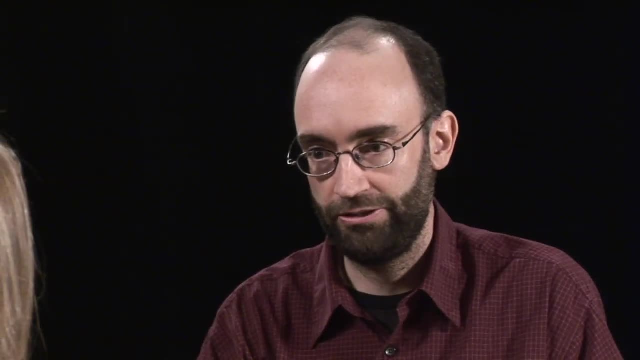 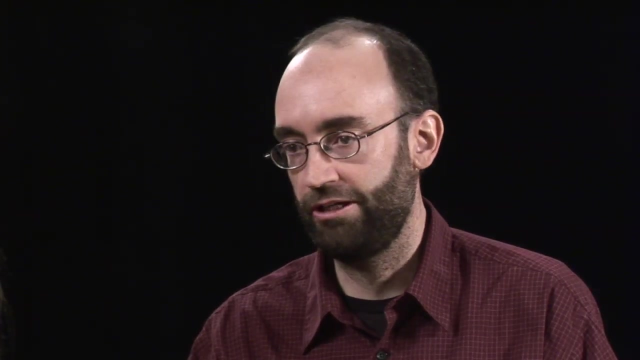 in this image is not being extracted. It's being extracted in B1.. So when I mentioned earlier that there were areas in higher visual cortex that are specialized for different kinds of information, whether it be faces or motion or whatever, there are areas in higher visual cortex that are specialized. 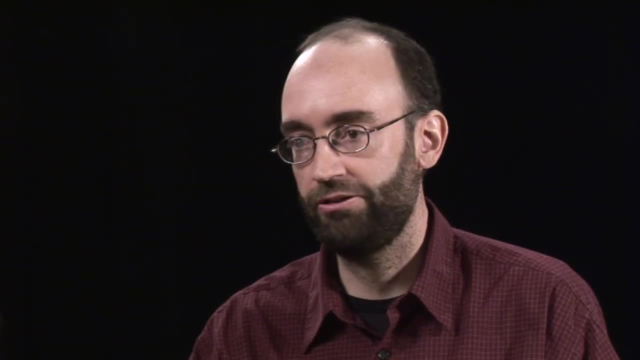 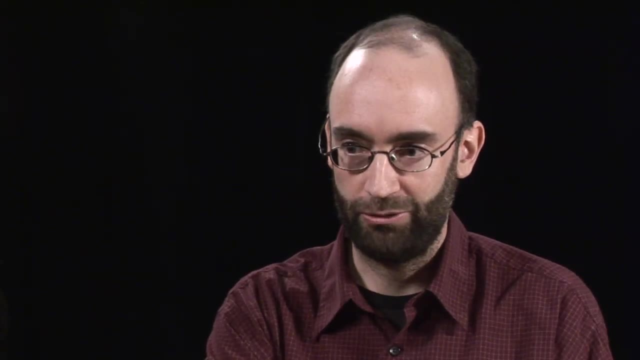 for extracting the 3D structure of scenes. So what we actually think is going on is that these higher visual areas are extracting the 3D scene structure and that's being fed back, through those feedback pathways that I talked about earlier, into B1, and it's after. 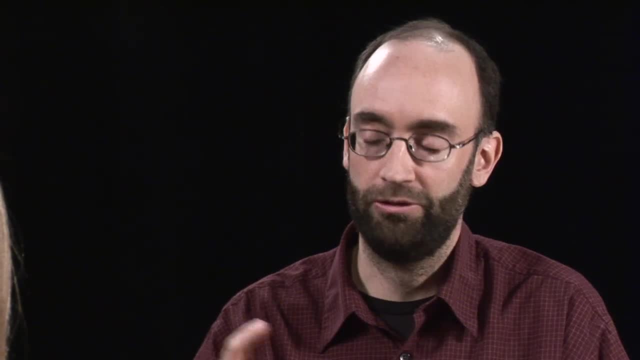 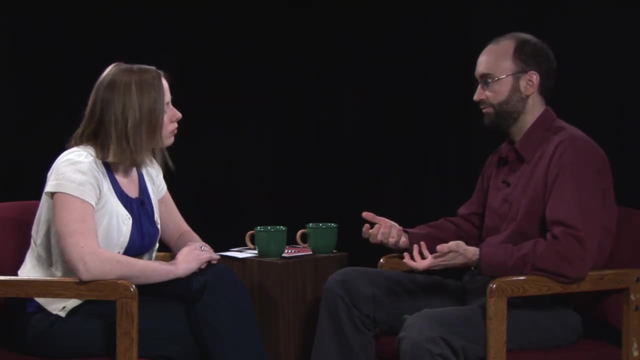 that feedback? The feedback happens is when the rescaling or the remapping in B1 occurs. So if you separated the representations in time, so for example there could be a veridical representation of the retinal information, that is to say in B1, early time windows. 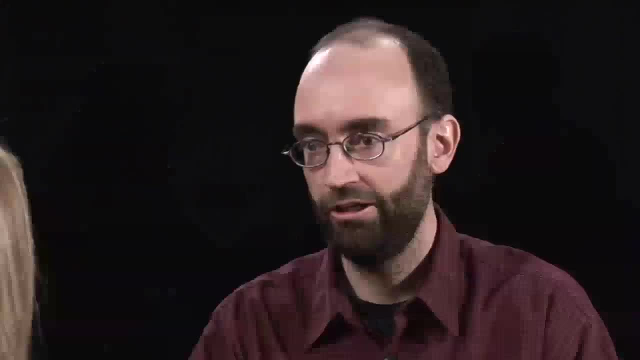 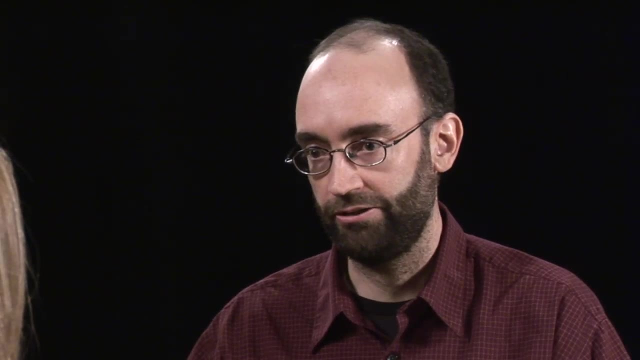 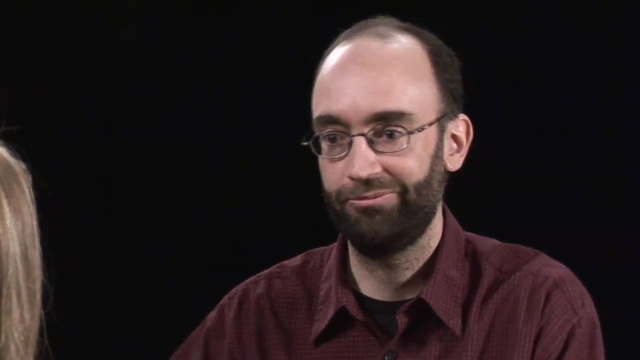 or early stages of processing in time could represent the accurate retinal information and then later stages, then integration. So that's what we're trying to do, is to replicate the 3D context and rescale it in the direction of its true environmental size, constancy direction. 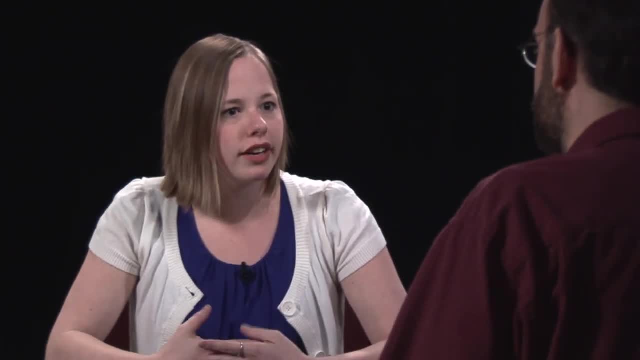 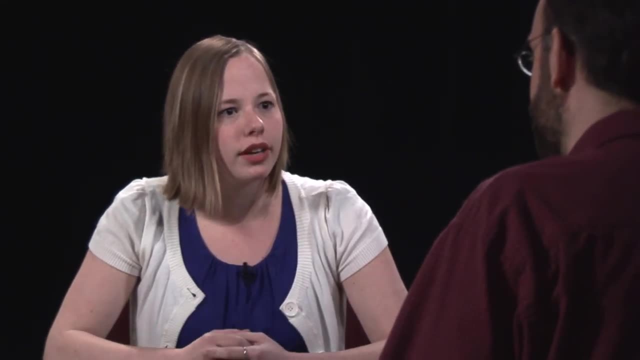 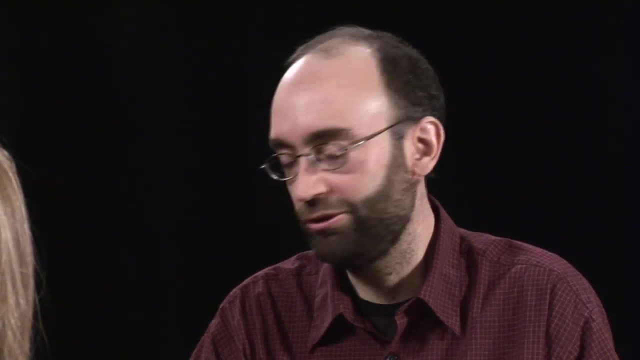 So now, as far as timing is concerned, you do your studies through fMRI correct? That's right, And fMRI tends to not have very good temporal resolution or timing, so how can you answer those questions Right? Actually, it has lousy temporal resolution and if we just use fMRI we'd not be able. 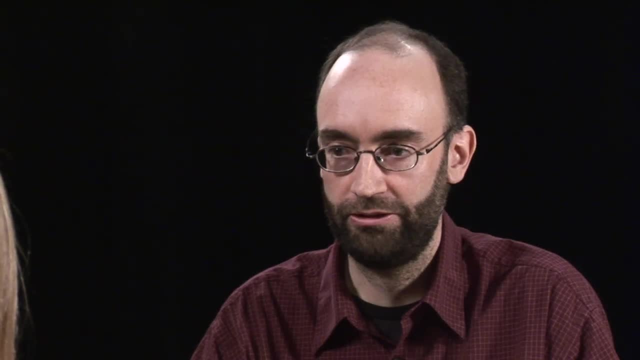 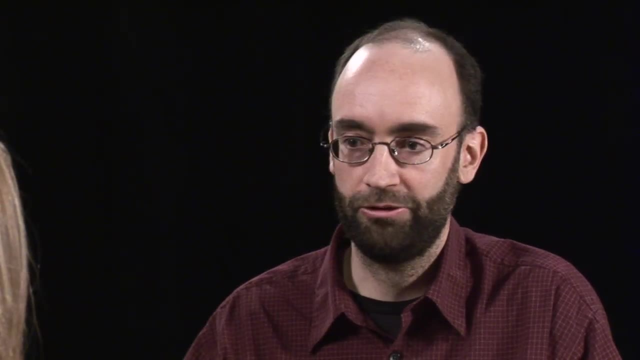 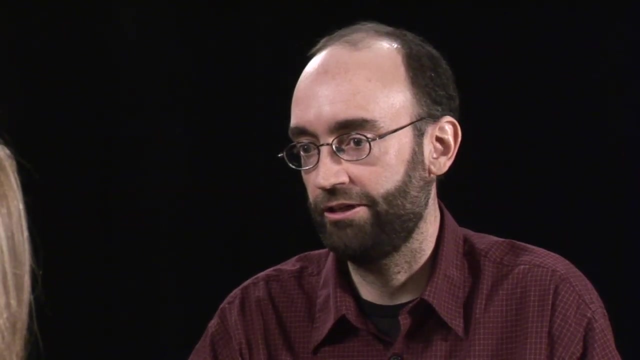 to answer that question. So what we've been doing is actually using scalp-recorded electrical potentials, or EEG or ERPs, with a very similar stimulus and asking when, temporally, do we see an effect? And actually what we're seeing is something like I described, so very early time windows. 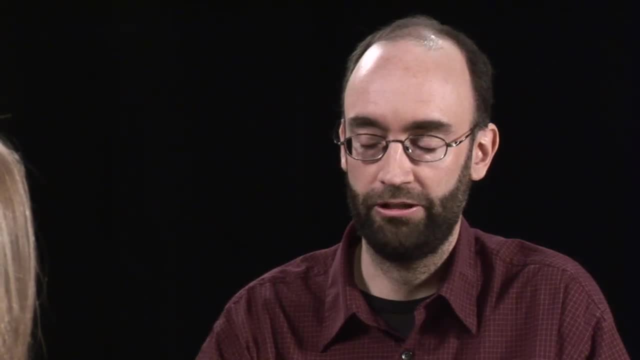 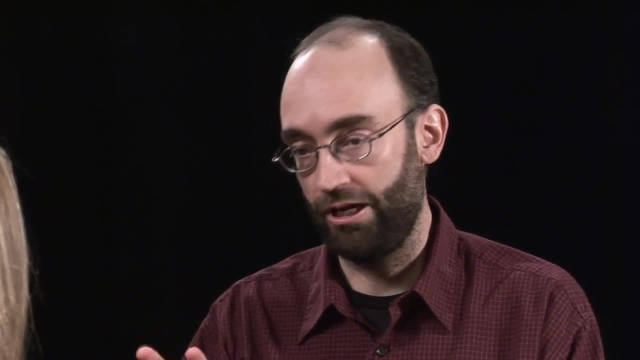 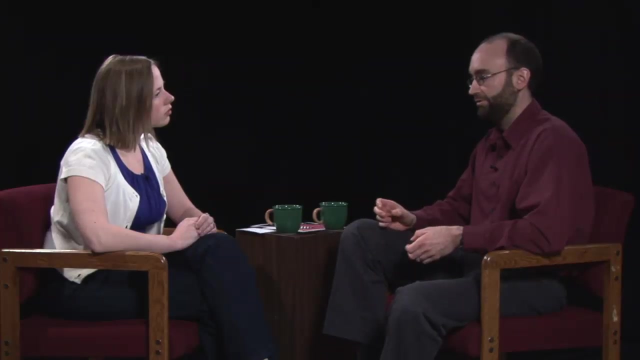 in the EEG response that we believe are being that are originating in B1, reflect the true retinal size of the retina, Okay, And then later time windows reflect the perceived size. What it demonstrates really is the overall importance of just of that transformation. 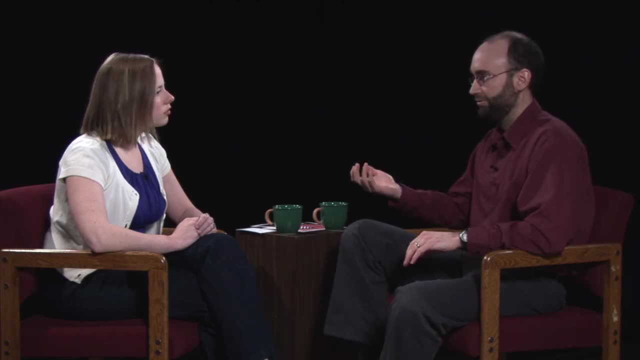 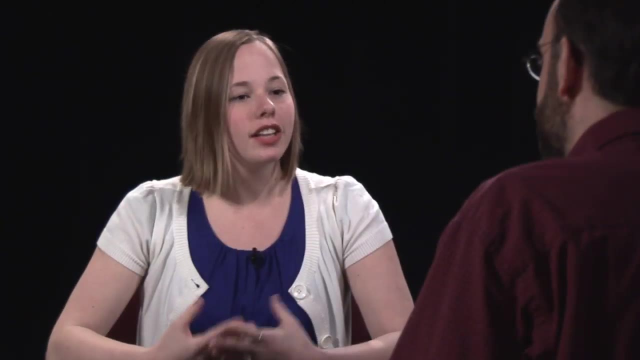 from the proximal to distal stimulus. That's what the visual system is trying to do, and it's trying to do it from the very earliest stages of the visual system onwards. In a lot of your experiments you're using actually two-dimensional elements. 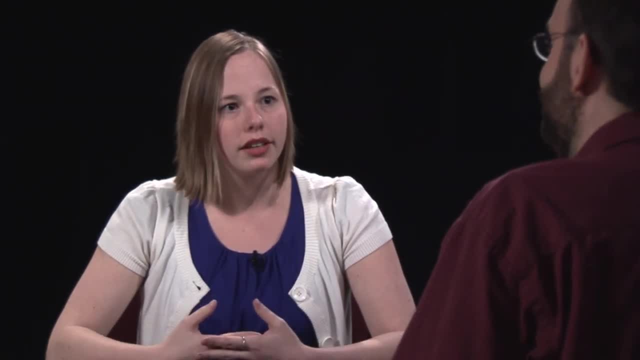 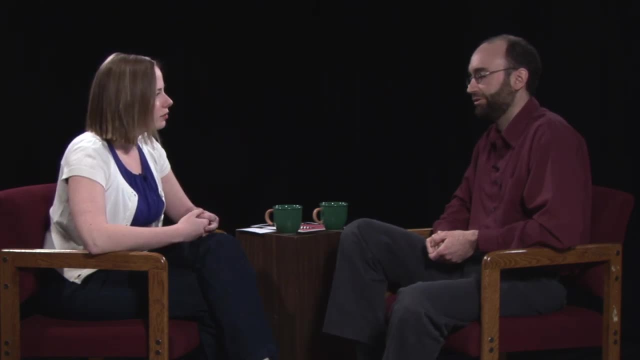 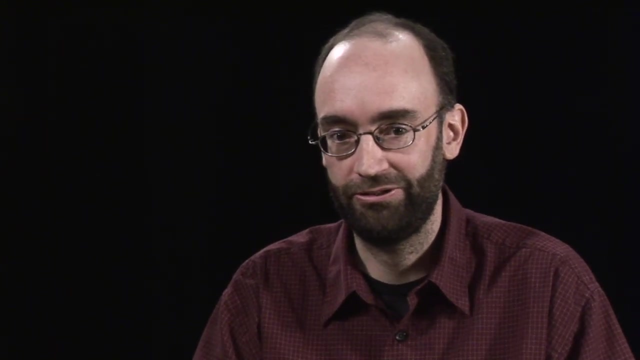 You're using two-dimensional stimuli that maybe has the illusion of being in three dimensions. What happens when we add in stereoscopic and other 3D visual cues to depth? Yeah, that's a great point. So it's really just sort of an experimental convenience that I use actually 2D stimulus. 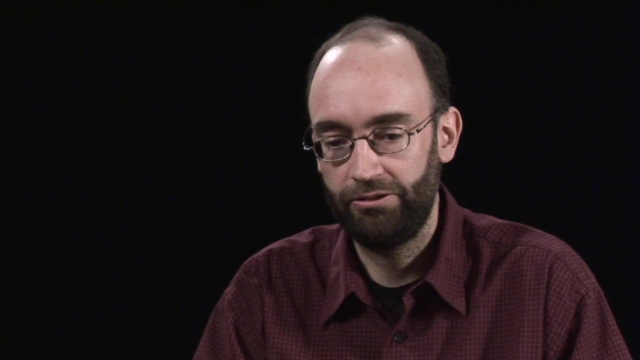 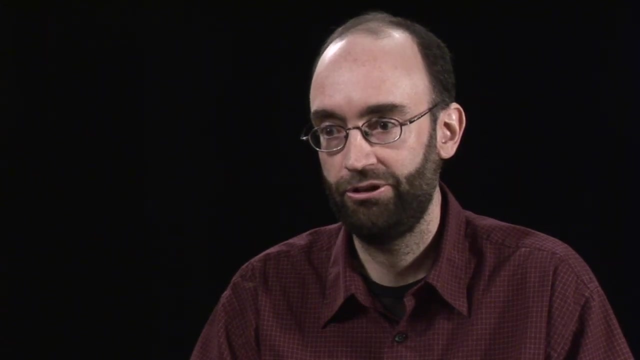 in which you perceive to be 3D, three-dimensional, I think, adding more cues. whatever those cues happen to be, if they happen to be stereoscopic, it's just going to make the effects even more obvious, Even larger and more compelling. 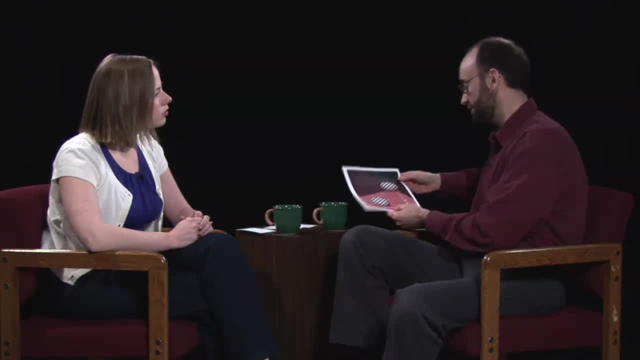 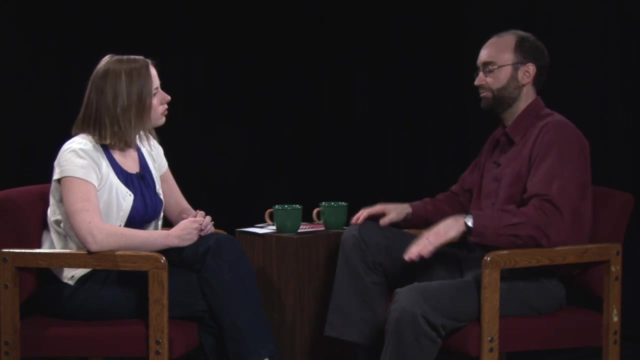 So, for example, if we take this example that we looked at earlier, even though most everyone will perceive these two spheres as being different sizes, if you make the cues more realistic by adding stereo, that effect becomes even larger. So I would presume that the effects that we're measuring, whether they be with fMRI or ERP, 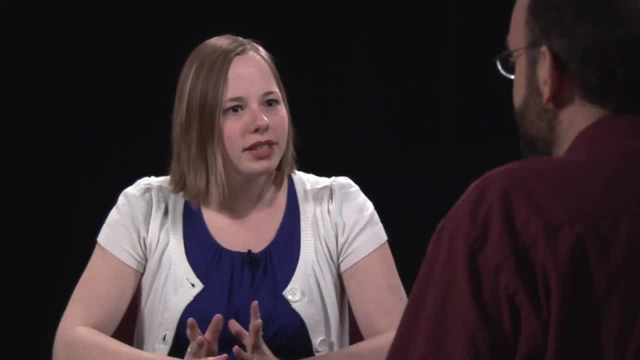 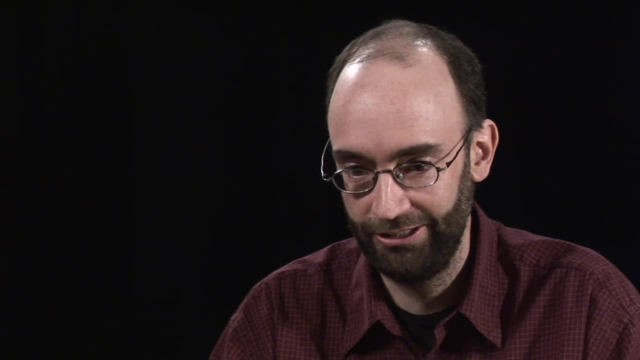 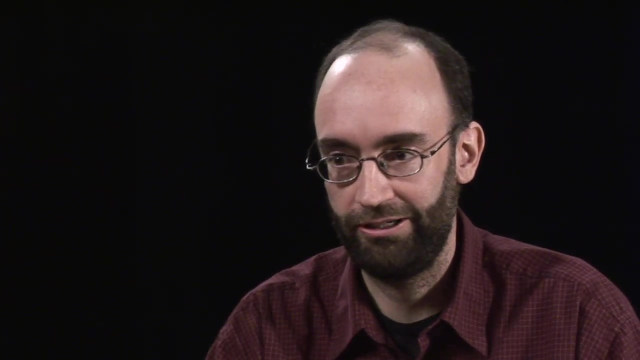 would also become larger as well. So what are the limits to this scaling that goes on? Yeah, that's a good point. So if we keep adding more and more cues and the effect gets larger and larger, is it the case that we could activate twice as much cortical area in V1 for one object versus 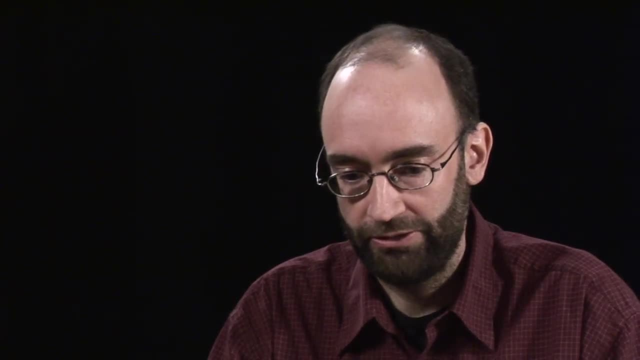 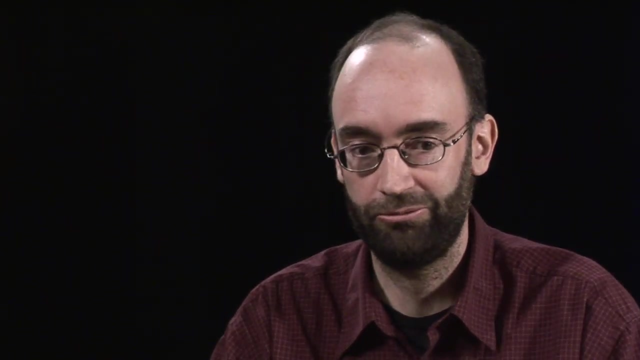 another. There are a couple points to consider there. First, size constancy as a perceptual phenomenon is not perfect. So, for example, even though you can recognize me as 6 feet tall when I'm sitting on the stage, I'm not going to be able to do a whole lot of that. I'm going to be sitting on the stage for the rest of my life. I'm going to be sitting on the stage for a long time. So I'm going to be sitting on the stage for a long time And I'm going to be sitting on the stage for a long time. 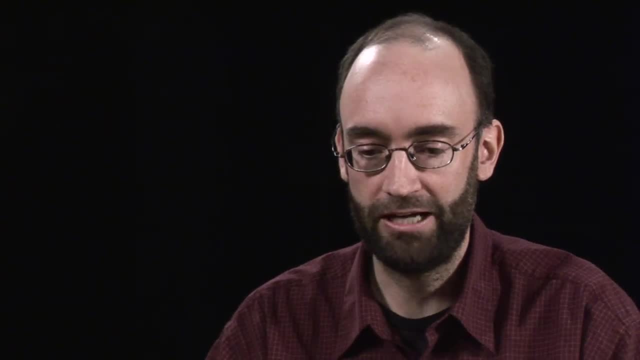 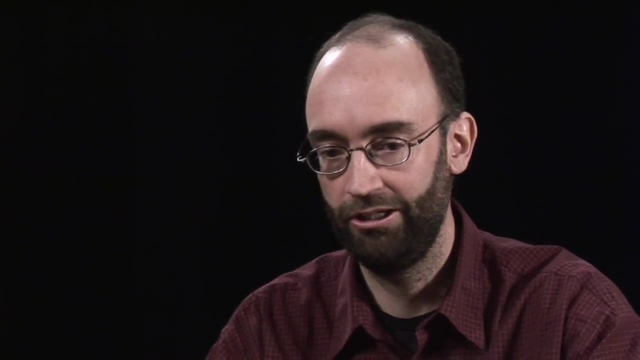 I'm going to be sitting on the stage for a long time. close versus far away, you still have access to the fact that the retinal size is changing. so if you look at a person who's across the parking lot, for example, you can recognize that you know they occupy of a fairly small portion of your 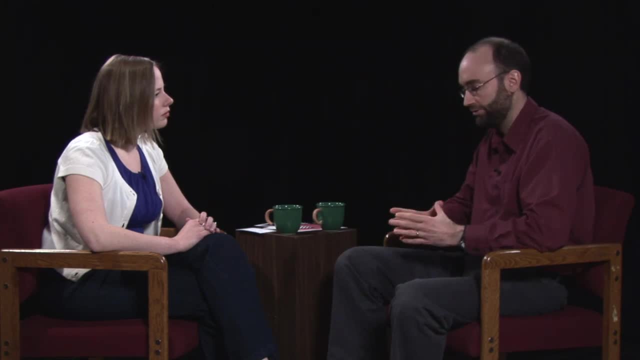 retinal image. and then the second part of that question really is how much these maps can change and that we don't know, and we're actually adding more and more cues to see at what point this phenomenon breaks, say in v1 and sort of what I suspect is that we have multiple visual areas. we have v1, we have v2, v3, v4. 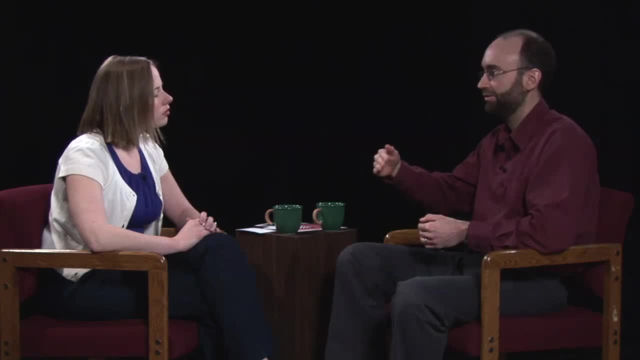 and I would expect that at some point v1 is no longer going to be able to rescale its representation, but possibly higher visual areas would start to reflect larger and larger changes. but that's you know, that's the way I see it. Now, what is the response been from your peers, since this is kind of really going? 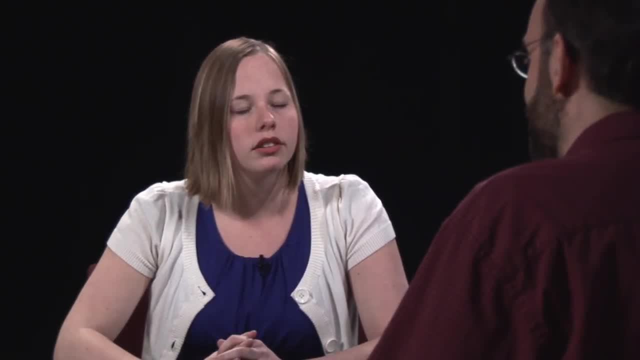 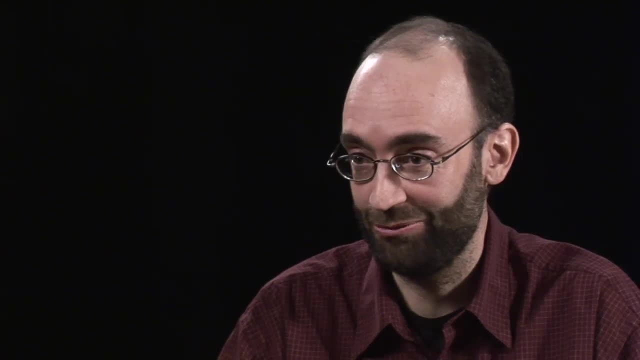 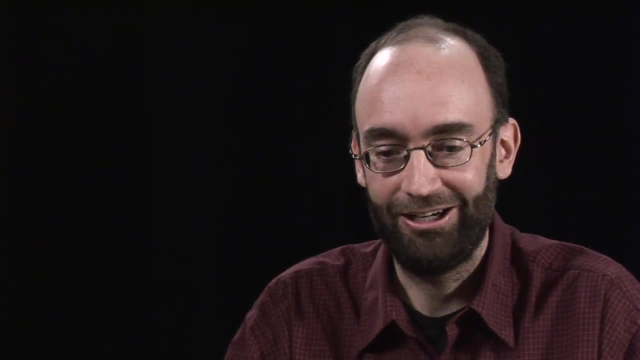 against what has been traditionally thought of v1 was doing. Yeah, it's going against what was traditionally thought. v1 was how v1 works. it went against the way I thought v1 worked. so, for example, this size illusion experiment really started out as a control experiment, where I was 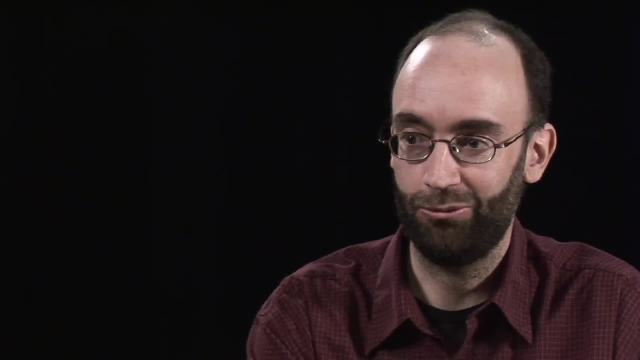 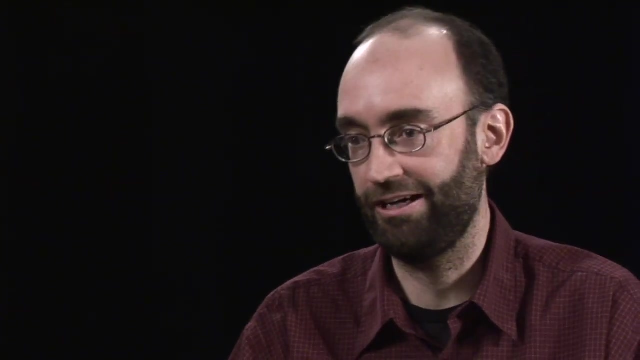 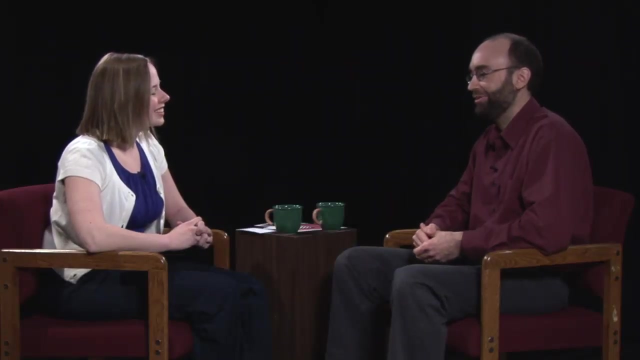 going to set out to show that at the level of v1, that these two objects would be, who would have the same representation. that was the point of doing that experiment, but in fact what I found was that it actually reflected perception, which was surprising and understandably it's been. 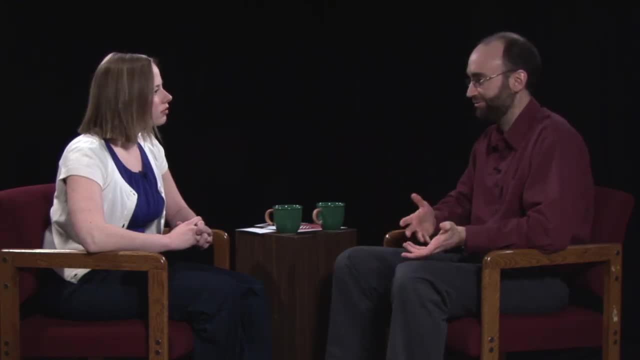 met with sort of a mix of excitement, because it's something new, and an understandable amount of skepticism as well, because what it implies are some fairly large changes at the level of individual neurons. so it's implying that in some circumstances- so for example when the sphere is small, that neurons aren't responding, and when the 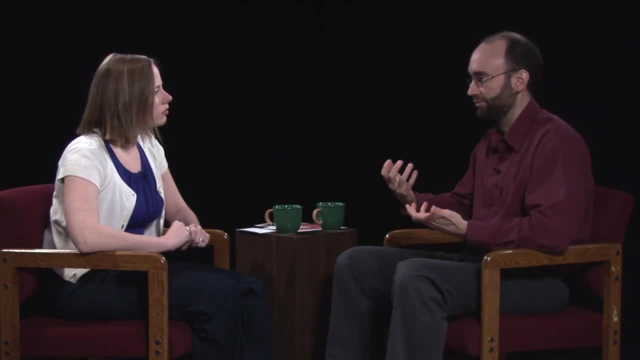 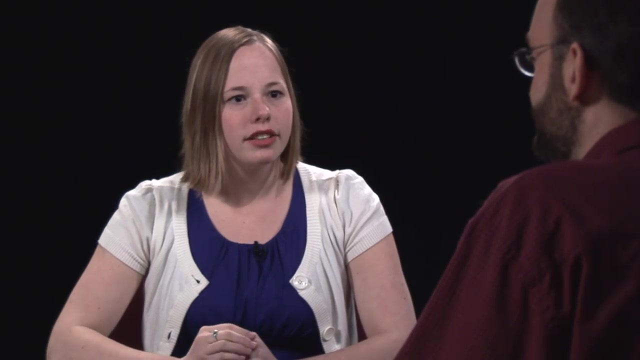 sphere is big neurons are responding, which is really a change in the receptive field properties of a neuron at very, very early stages of the visual system, which is surprising. so what do you think needs to be done for this to be a generally accepted idea of how v1 works? 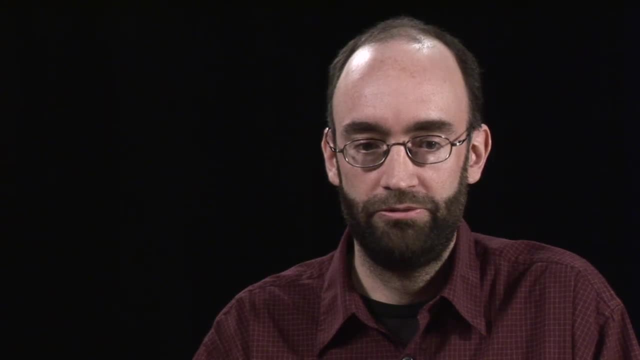 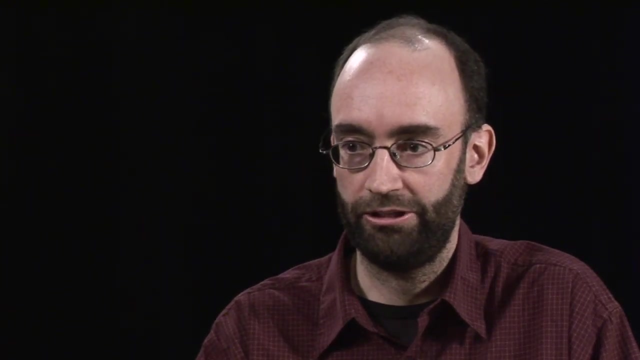 well, I think what we really need to do is get data at the single unit electrophysiological level. that is, what are single neurons doing to this perceived size difference? because it implies that receptive fields are changing, that is, in some circumstances they are responding to a visual stimulus and other. 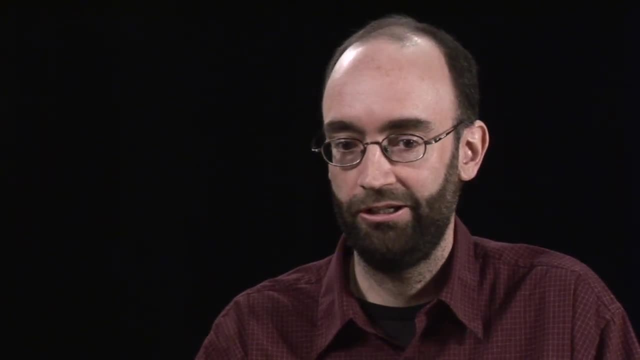 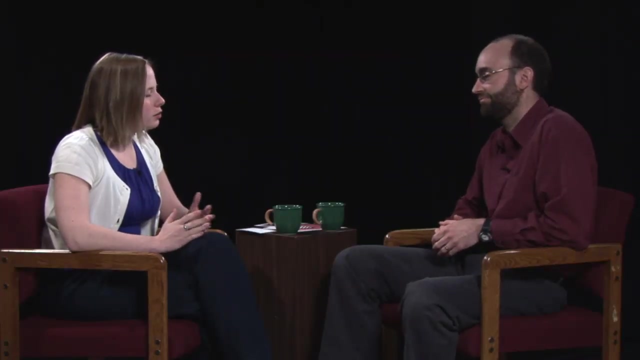 circumstances are not, so we have to actually go in and measure single neuron responses in v1. so do you have a position then on the two opposing theories, of one being more problem-solving way we process information versus the gibsonian approach to bottom up that our visual field has all the information we need? 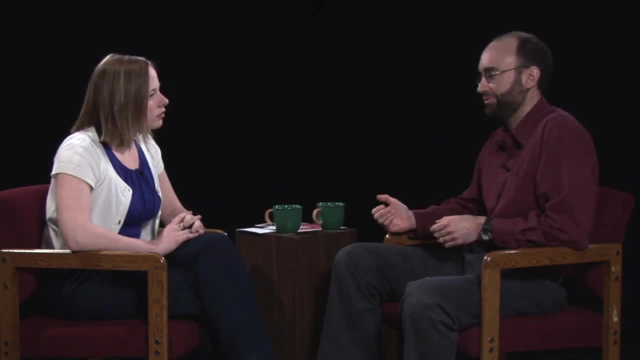 right. so one might be tempted to think, based on these results, that v1 is reflecting the size illusion. you might think that, like we kind of mentioned before, that v1 has done everything, that all the information is there, present in the image and boom, it's done by v1. but actually it's. 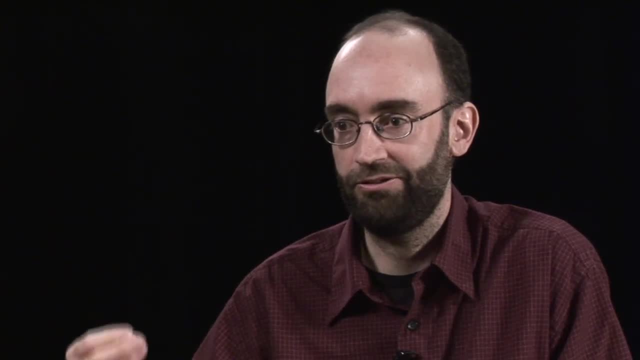 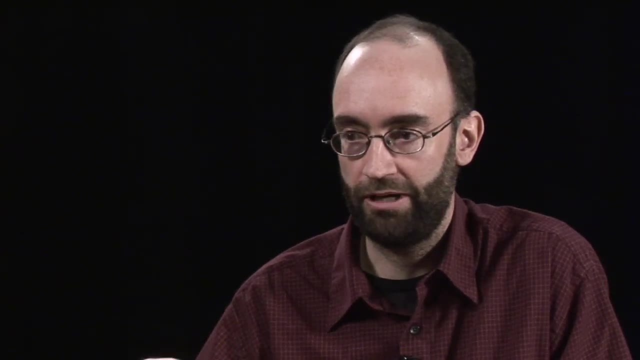 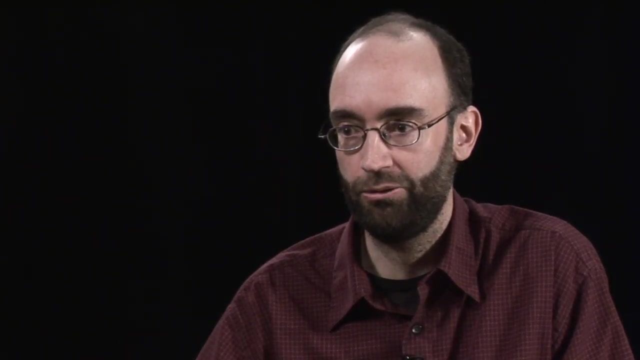 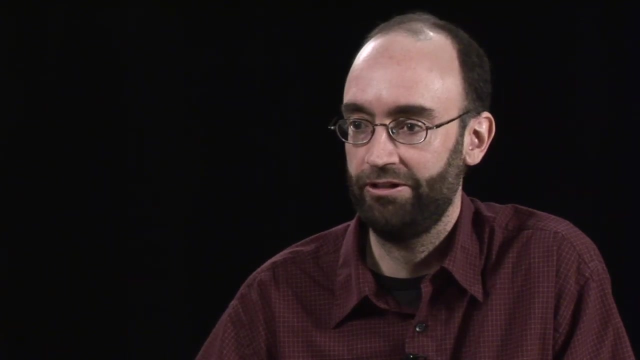 important to remember where this source of the information is coming from to mediate the effects in v1, and I really think that it's it's being derived from higher visual areas that are extracting the 3d contextual information. so I think it's actually more in line with sort of the Helmholtzian view, that of an inferential process, that 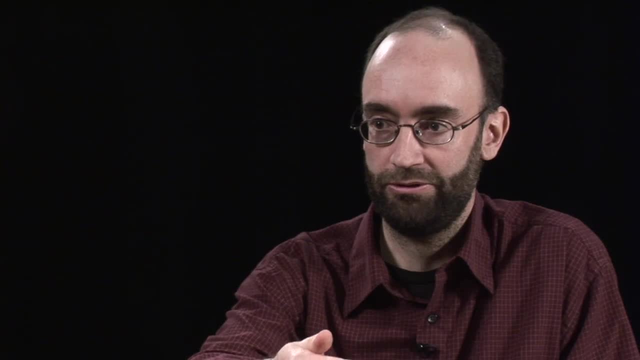 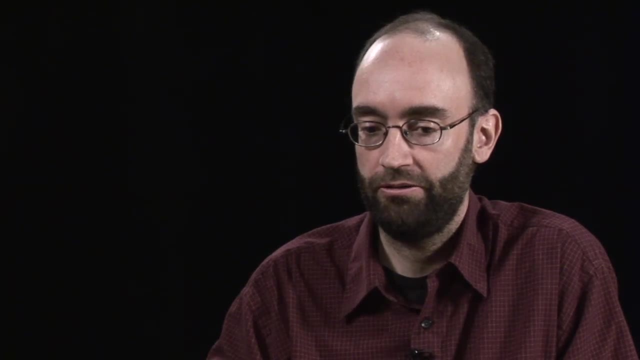 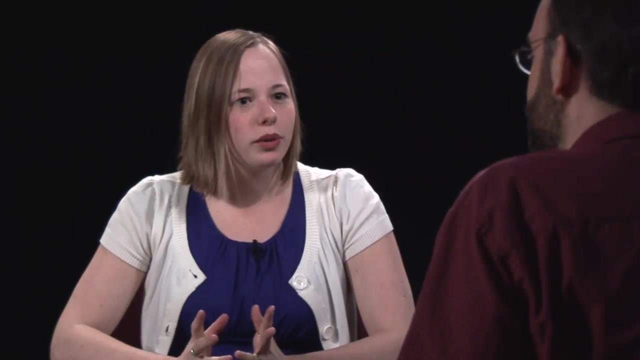 the visual information is trying to infer what's out there in the visual world through the use of contextual information, and it's it's that inferential process is being reflected in the activity patterns in v1. so, in your opinion, what do you think are some of the main big unanswered questions that 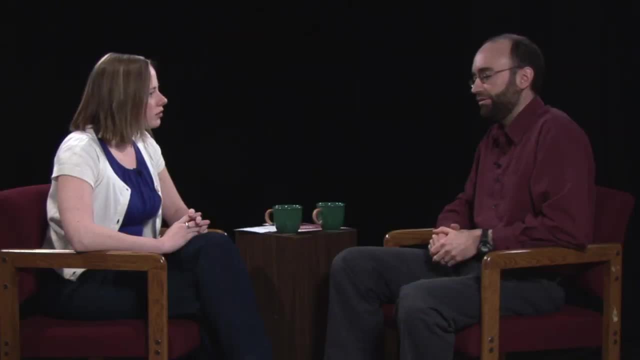 you'd like to see answered in this area. well, we have a pretty good understanding of how lower visual areas work. so, for example, we think we know generally how v1 works in terms of what kinds of visual information it responds to the fact that it is modulated by contextual 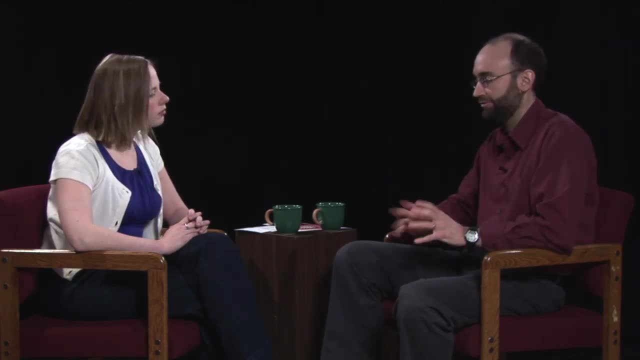 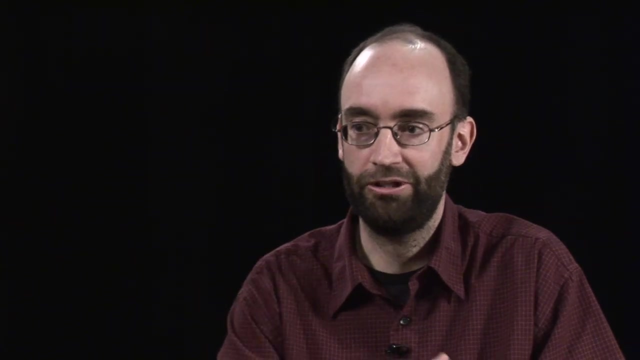 information is surprising, but overall we have some idea of how it works. we also have some idea of how higher visual areas work, such as areas that are specialized for processing faces or locations or motion. but where we have a really poor understanding about are those intermediate areas. those areas- 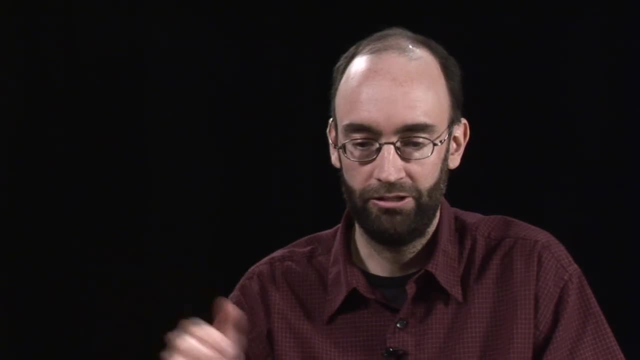 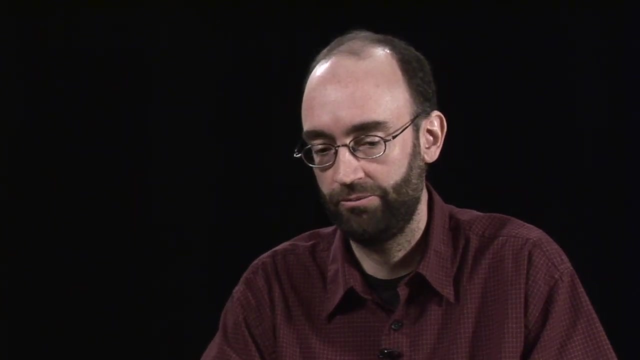 between v1 and v2 and the higher stages of the visual system. So, for example, we have very little understanding of even how V2 works, the very next stage of visual processing after V1.. And I think what's going to be required is some new thinking. 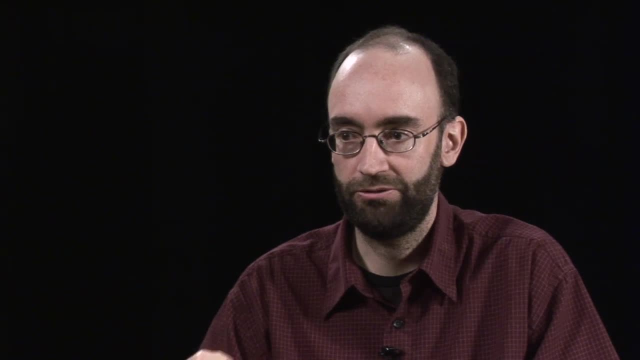 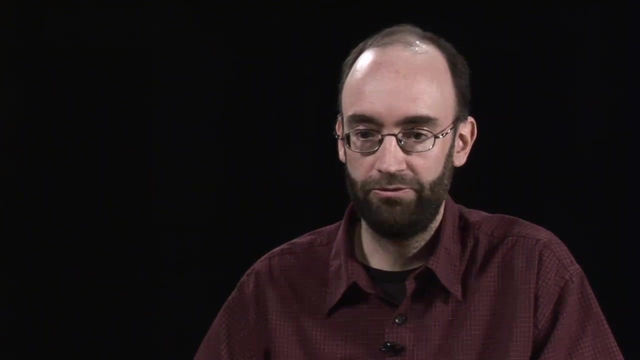 in terms of what it is our visual system is trying to achieve, And I think what these experiments- so, for example, what the size experiments are good for- is actually just challenging the traditional way of thinking about the visual system as a feed-forward hierarchical system. 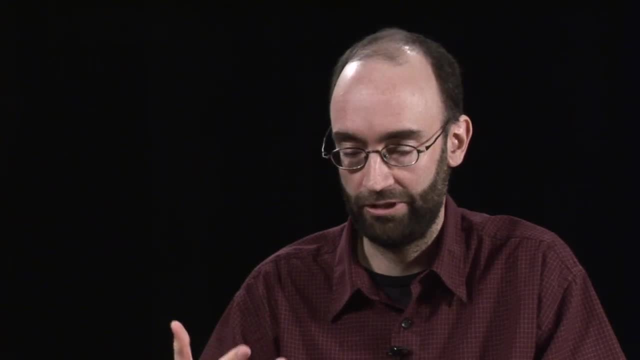 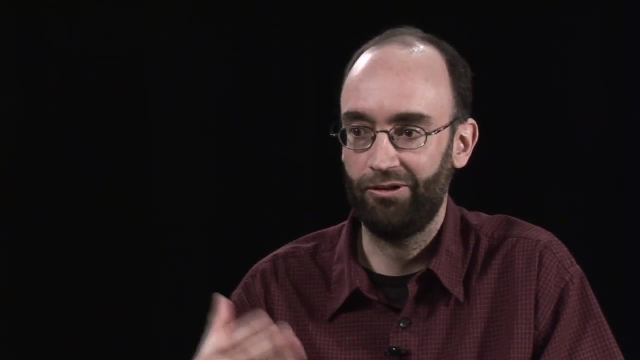 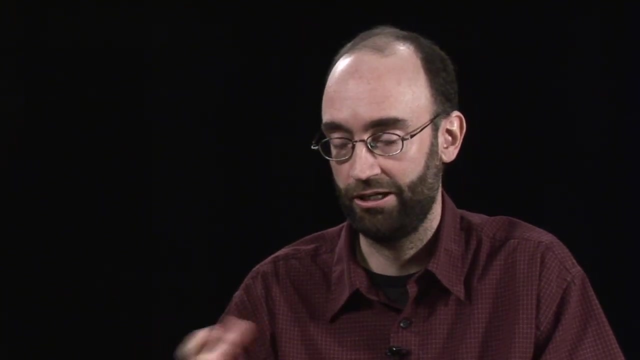 and remembering that feedback processes are going to have a large influence. But beyond that, we're going to have to be, I think, more creative in thinking about what it is these different visual areas are designed to do within the context of visual processing. 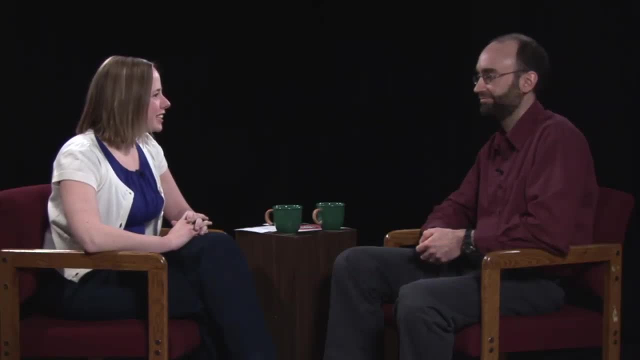 Thank you very much, Dr Murray, for having time to speak with us today. We really appreciate it. It was my pleasure. 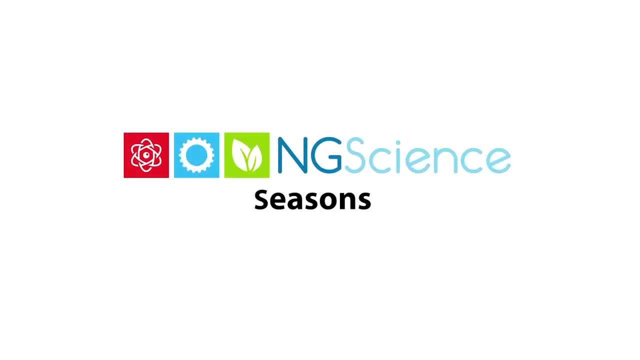 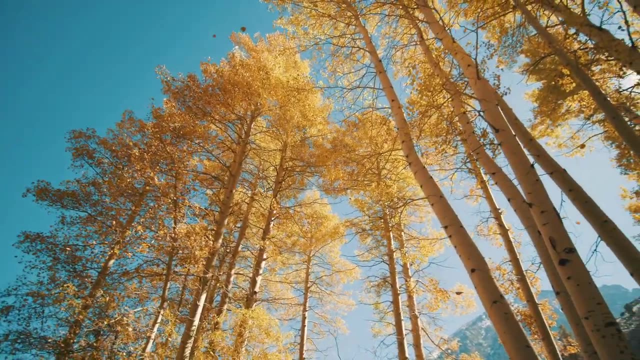 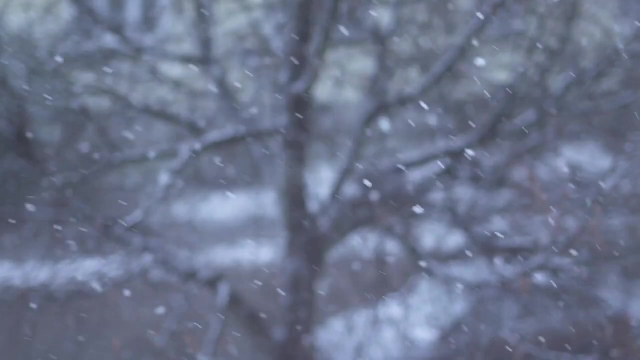 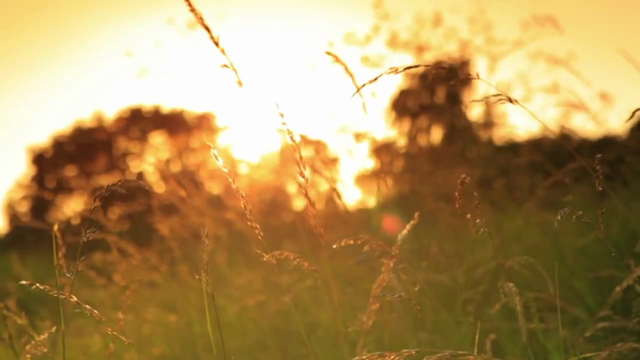 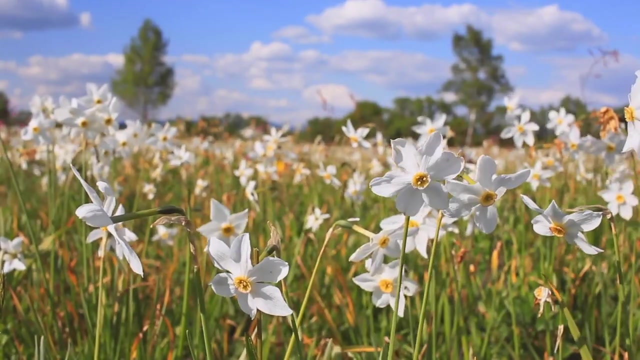 You may have noticed that the weather changes a lot throughout the year. In some months the days are short and it can get pretty cold. It might even snow. In other months there are more hours of daylight. It can be sunny and hot almost every day. 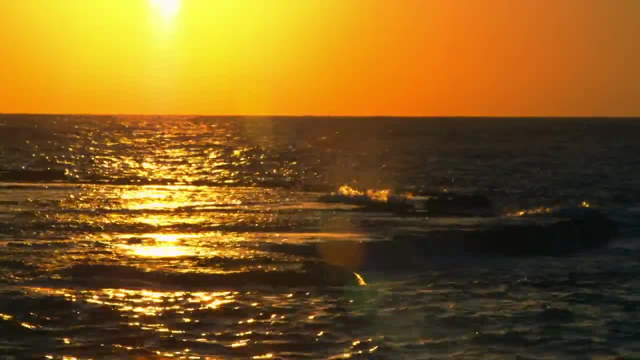 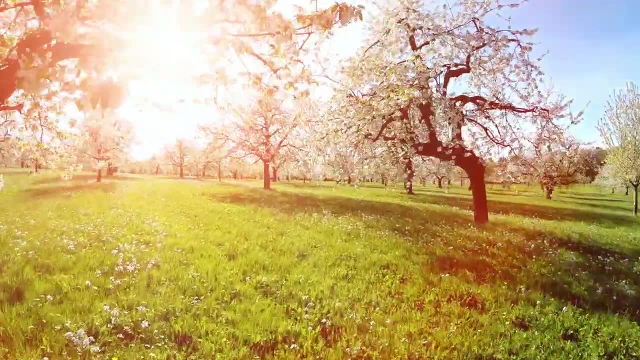 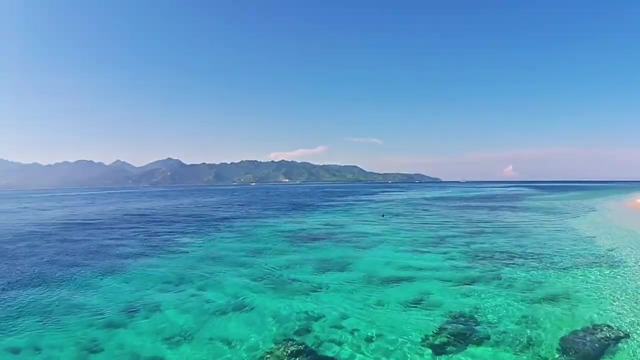 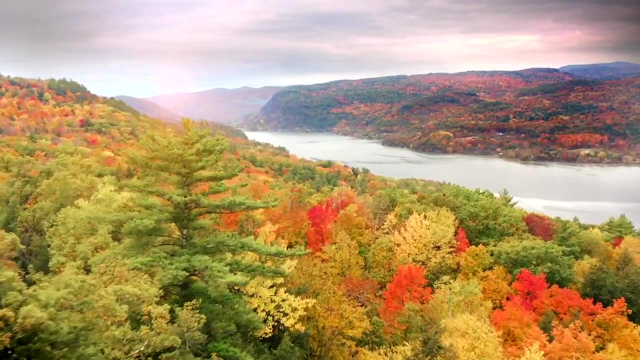 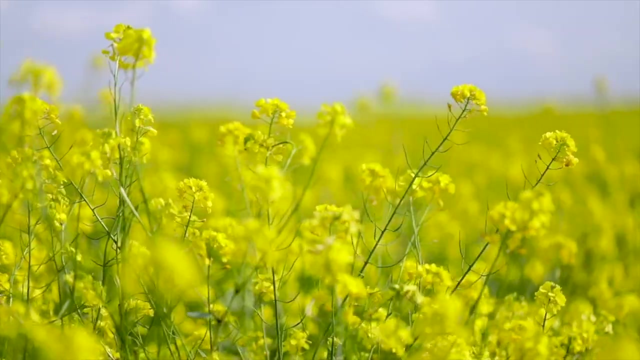 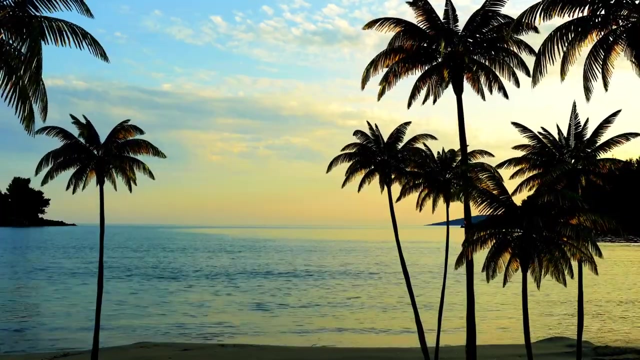 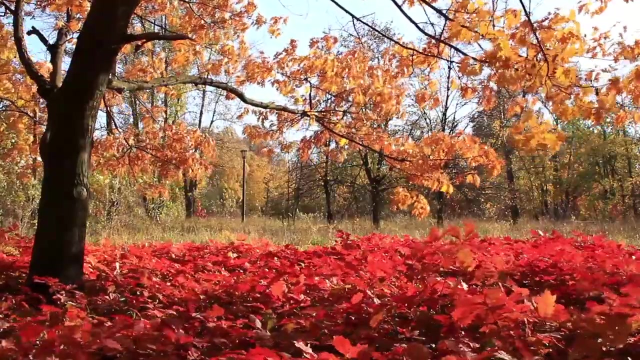 These yearly weather patterns are called seasons and they occur due to the position and movement of the earth around the Sun. There are four different seasons: Summer, autumn, winter and spring. Summer is the hottest season, with the most hours of daylight. As summer moves to autumn or fall, the weather gets cooler and there are fewer. hours of daylight. At least we can see this if you are caught in a closed, closed way. These are the three seasons the seasons will affect. The above are know forienie Christmas season. Those coming up are 여러분's feelings in a winters season.